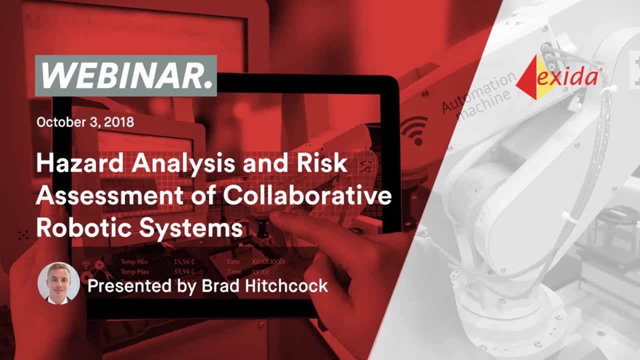 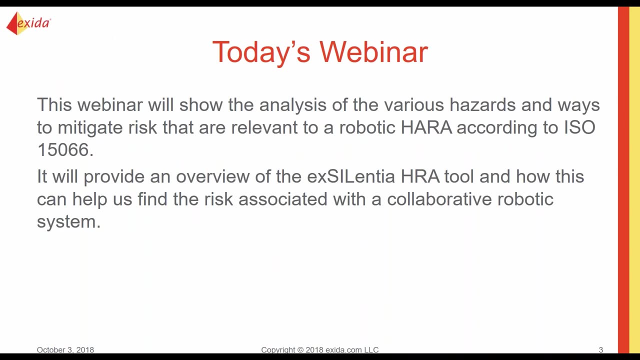 Okay, I think we're ready to start. So today's webinar is going to be on hazard analysis and risk assessments of collaborative robots. So this webinar is going to show the analysis of various hazards and ways to mitigate risk relevant to ISO 15066,, which is a supplement in support to ISO 10218,, which provides 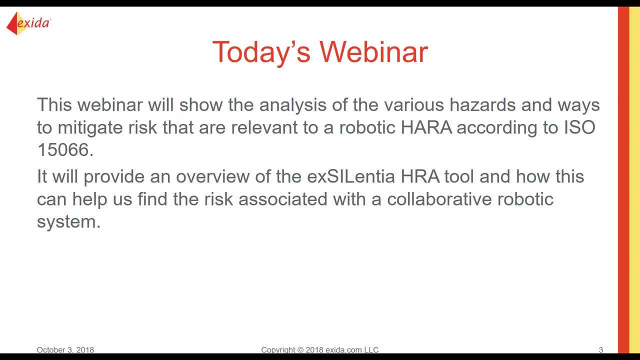 industrial robot safety standards And this is going to specify more geared towards collaborative robots. This webinar is also going to provide an overview of the Excellencia HRA tool- hazard risk analysis- and how this is going to help us organize and find our risk associated with collaborative robot systems. 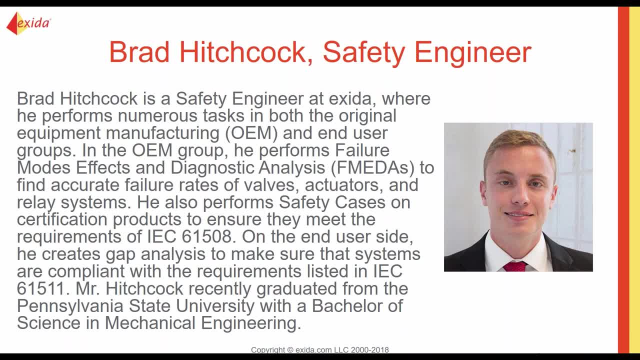 So my name is Brad Hitchcock. I'm a safety engineer at Exeda. I work in both the OEM group, which does certifications of final elements, and I also work with the end users. where we'll be focusing here includes the collaborative robots. I do gap analysis. 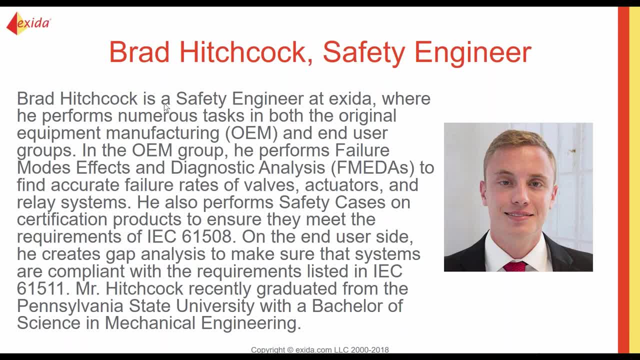 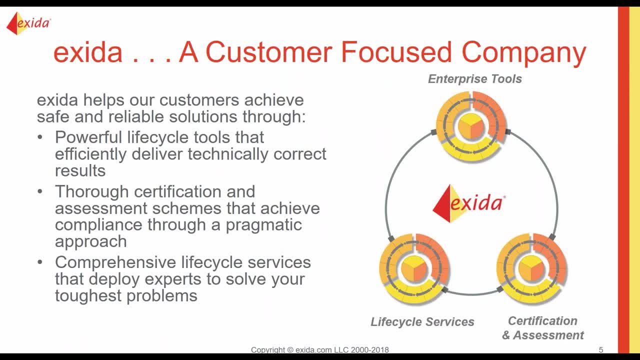 and I also work with the technical team to make sure that systems are compliant with 61511.. So Exeda helps our customers achieve safe and reliable solutions through just knowing the safety lifecycle and our tools. So we use Excellencia to help us go through the safety lifecycle and 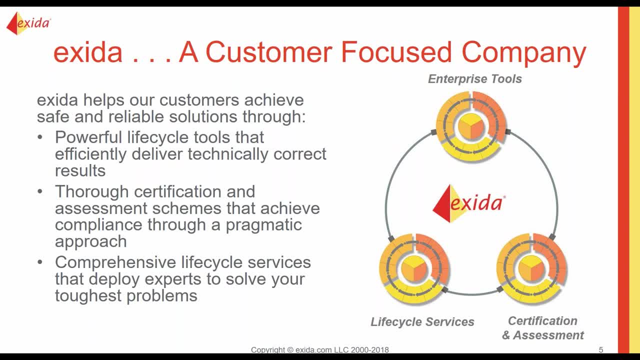 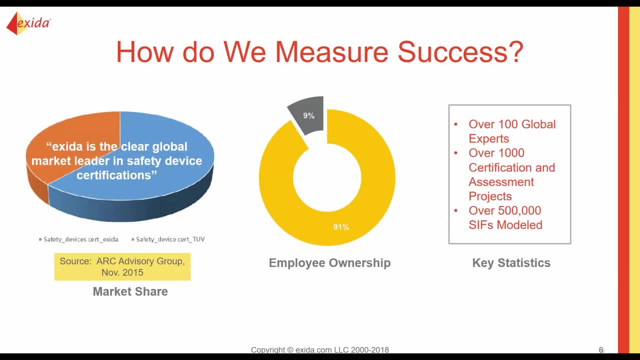 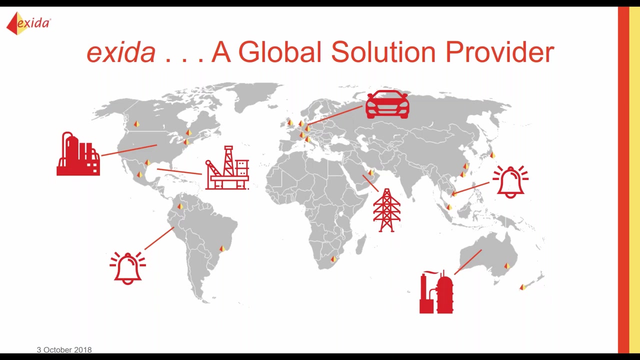 mitigate risk in systems and we also work in certification. So, as I said, with final elements and making sure they're compliant with IEC 61508. so we're actually the clear global market leader in device certifications. as you can see, we have two-thirds of the pie and we're also a global company. we work. 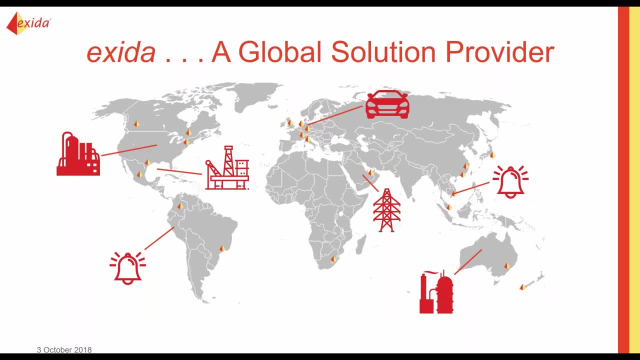 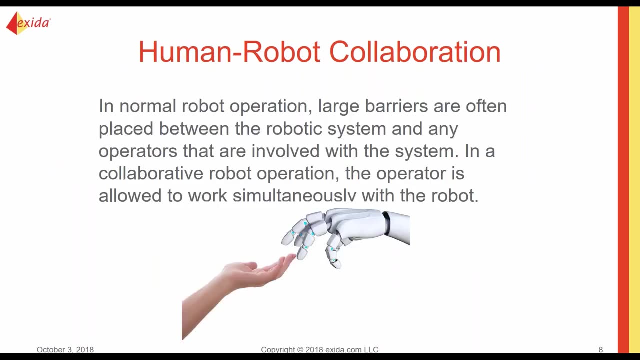 all over the world. our headquarters are in Sellersville, Pennsylvania, and in Germany, but we have locations that are everywhere and do various needs in alarm safety, cybersecurity and functional safety. okay, so what is human robot collaboration? so in our traditional industrial robot applications you have, you're gonna have large barriers that are placed between a 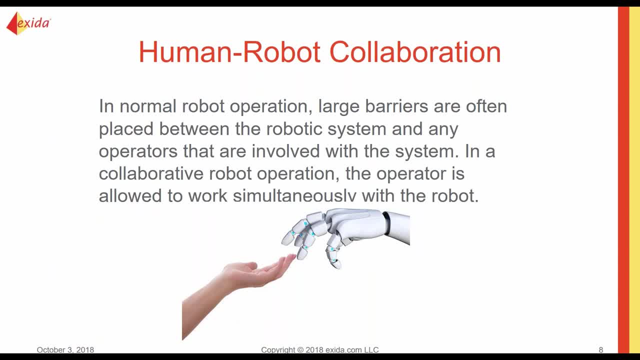 robotic system and the operator and they have to shut off if a robot wants to enter the air. you're gonna have large barriers that are placed between a robotic system and the operator and they have to shut off if a robot wants to enter the air, the workspace, while the collaborative robot allows us to simultaneously be in. 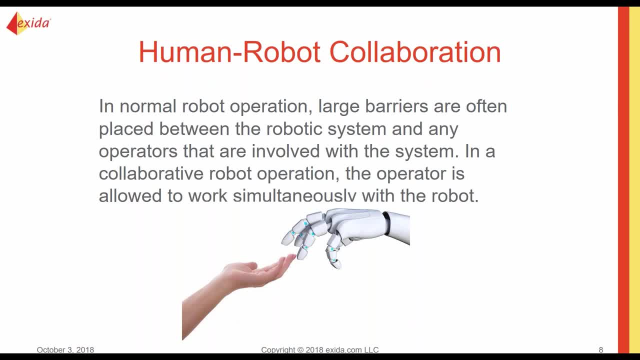 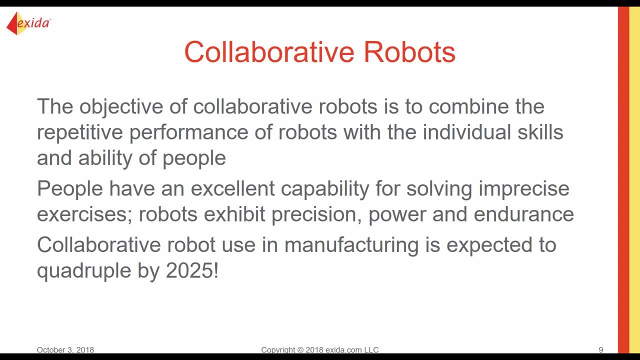 the same area with the robot and just create better efficiency. so the objective is to combine the repetitive performance of robots- so just doing monotonous tasks that humans won't want to do, or physically or physically demanding for people to do- and it combines that with precision and thinking of. 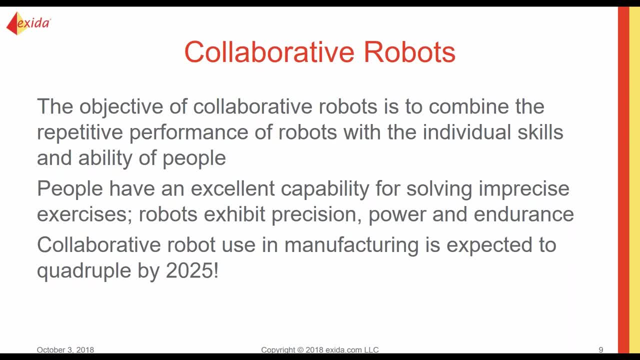 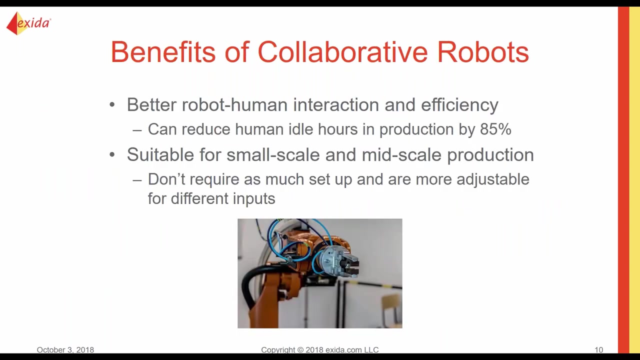 human beings. so collaborative robots in manufacturing will hopefully quadruple by 2025. so it's important that safety is in. their collaborative robot is keeping pace with the growth of the industry. so here are some of the benefits of collaborative robots. so there's better robot human interaction and 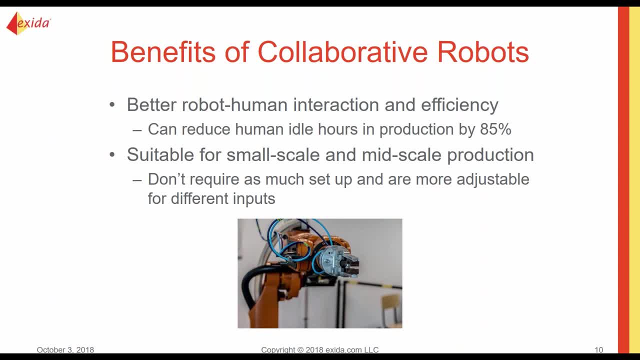 efficiency. so during a normal industrial robot application, whenever human intervention is required, the entire production needs to stop for the operator to enter the area, while the collaborative robot allows us to interact, and this will reduce the human idle hours in production by 85%. in addition, it's suitable for a small scale. 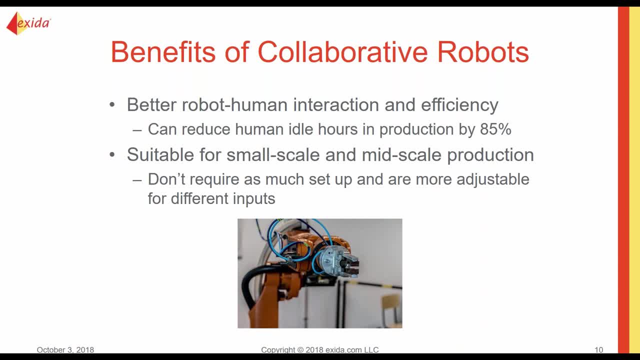 and mid scale production. so the current industrial robots: they're mainly only used for the large scale production because of enormous costs that go into buying large pieces of machinery and the complexity that comes with setting up and adjusting these large pieces of equipment. so it's really only going to be used for manufacturing where the same 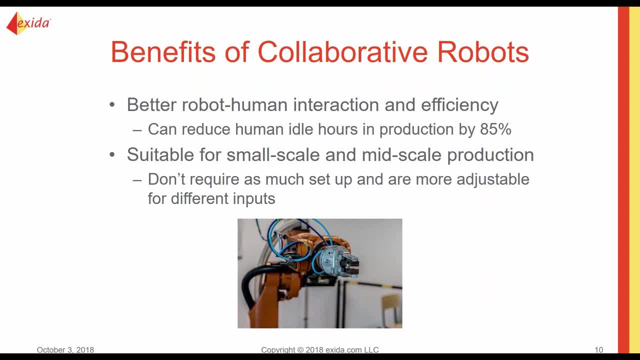 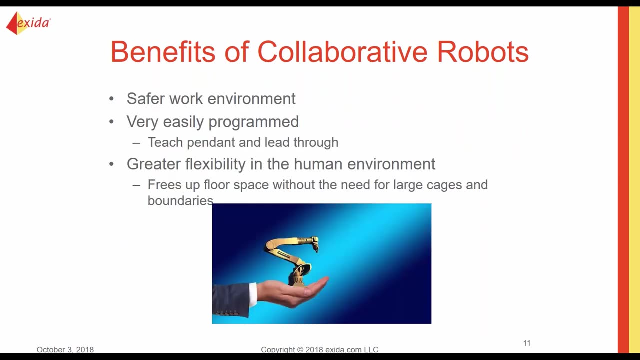 thing is being made just all day, every day. but with the collaborative robots they're easily set up and adjusted so that you can use them for multiple applications and are better for the small scale and mid scale production. so some more benefits of collaborative robots include it will. 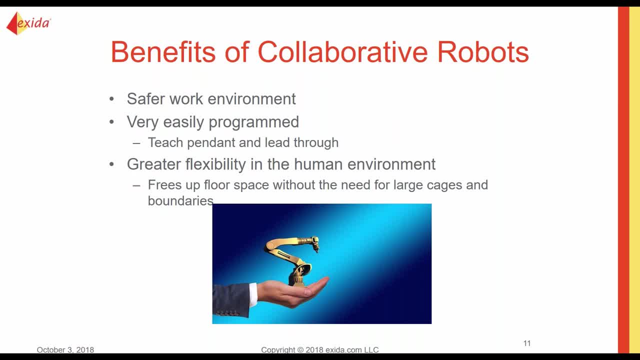 provide a safer work environment. so, since ISO 15066 is, it takes human involvement and collaboration in mind. compared to ISO 102 18, everything is just checked extra thoroughly for safety so that the robot will be- or the robots tend to be- much safer than the other robots. that make the work easier for the robots and the robots. take that: muchrodığ baking products in regular附. 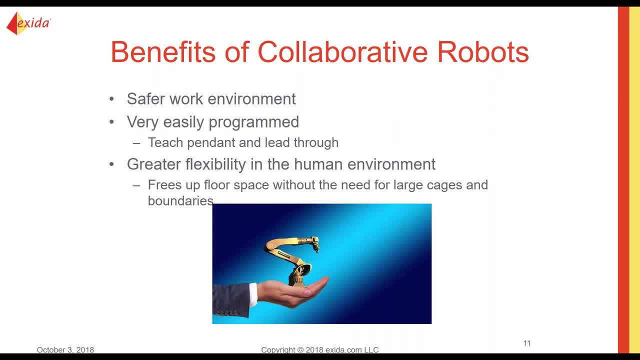 industrial robots Also, they're very easily programmed. so for the industrial robots you're going to have some complex coding that goes into programming the robots, while the collaborative robots they'll use teach pendant, which is basically you have a touchpad and you're gonna with the touchpad, you're just 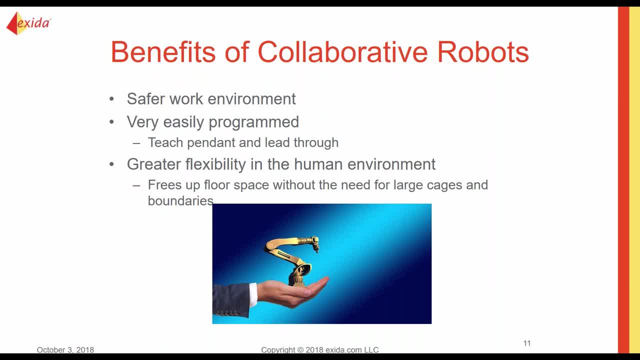 going to take the robot through different coordinates and the robots going to follow this when it goes in through its operation, and after that you can change different speeds, just so it's not going at the slow speed that it takes to program it at. Then there's also lead-through programming. 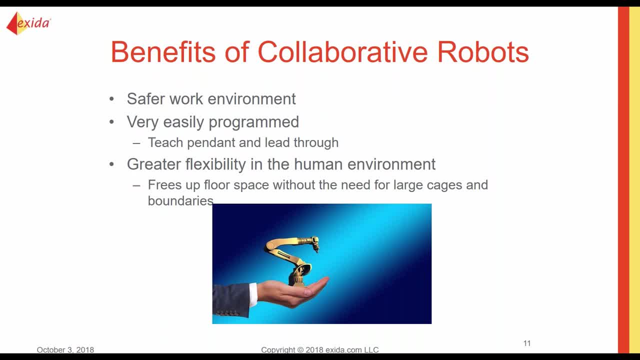 which is where the operator physically moves the robot to where the path of the robot needs to go, and it'll memorize that path and follow it. Last, there's greater flexibility in the human environment. so, since you don't have these huge gates that are protecting the robots from humans, it frees up a lot of. 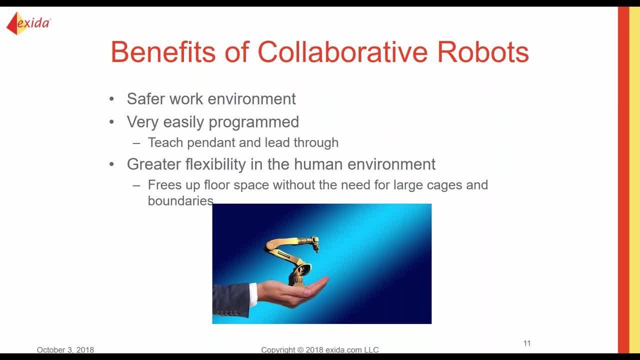 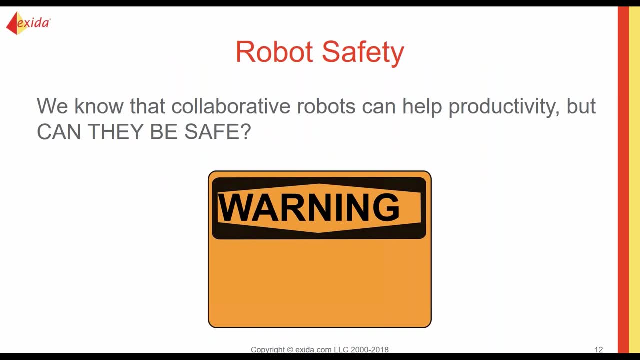 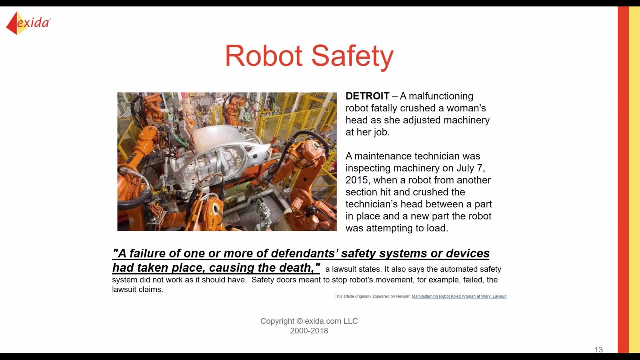 space in the workspace. Okay. so these collaborative robots, they're acknowledged to be very beneficial to manufacturing, but the question we need to really ask is: can they be safe? So here's an industrial robot application where a maintenance technician was inspecting machinery And a robot from a completely different section crushed the technician's head. 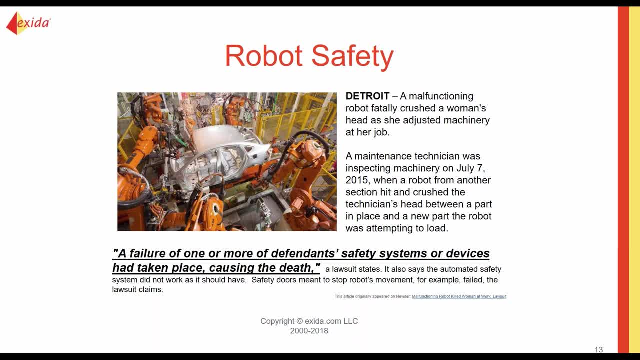 between a part in place and a new part. The robot was attempting to load and killed the operator. So when a death in an industry occurs, just huge safety concerns are naturally going to come up, and it's important that these are addressed and that if they can't be fixed, then the production can't go on. 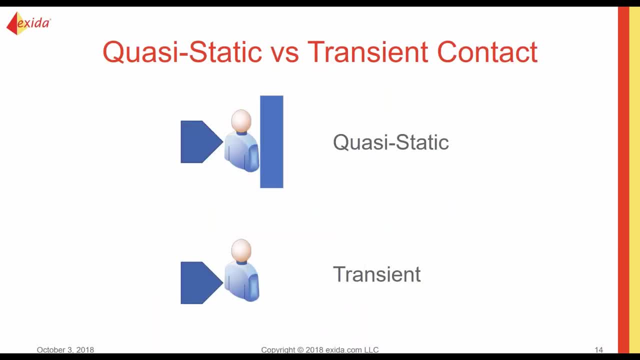 Two very important distinctions that we're gonna need to know about during this presentation when analyzing hazards and risk is the difference between quasi-static and transient contact. So in quasi-static contact you're gonna have an operator body part that is pushed up against a fixed surface by the robot or 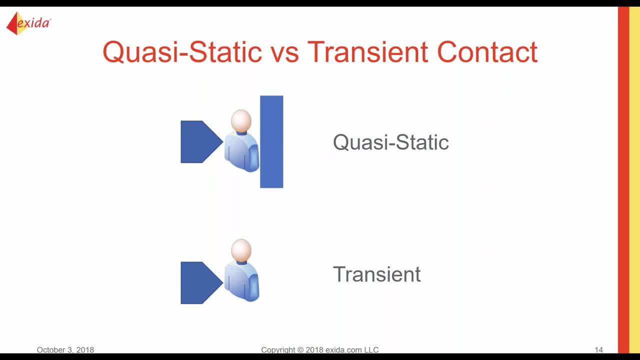 by any other moving machinery And this will make it so the operator can't move away from the hazard, for there's like a thrush a it's point. if it's more than 0.5 seconds that the operator can't move, then it's considered quasi-static, While transient is when the robot arms 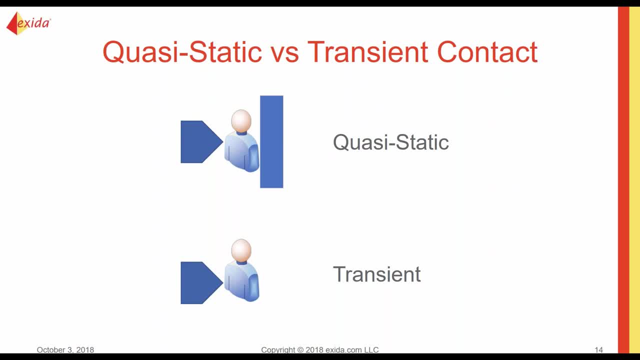 going to hit the operator in free space and the operator can immediately get away from the hazard. So the importance of this is, in quasi-static applications, the tolerable pain threshold- we're gonna talk about those later. it's going to be half as much as the transient, so it's very important. 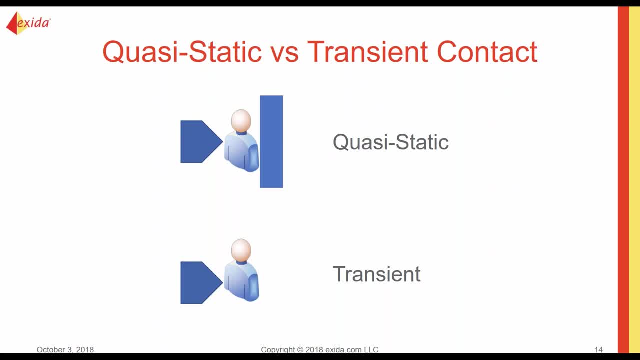 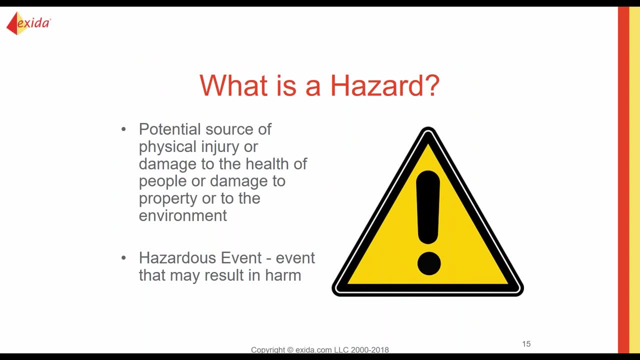 that quasi-static contact is avoided at all costs. So before we get into hazards and risk, we're just going to kind of go through some definitions. What is a hazard? It's a potential source of physical injury or damage to the health of people, or damage to property, or 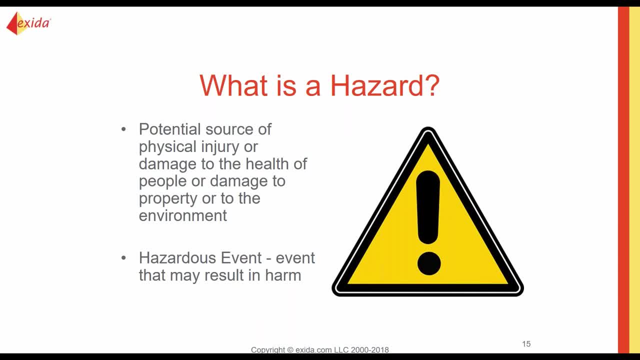 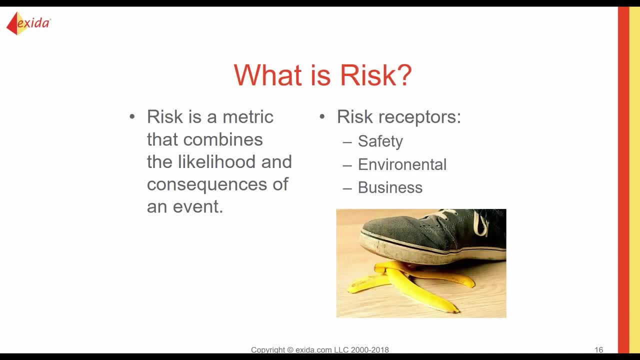 to the environment. A hazard event is an event that may result in harm and what is risk? So risk is going to look at your likelihood and consequence of an event and when you multiply those together you get your overall risk. So this is important with safety risk. so an operator being 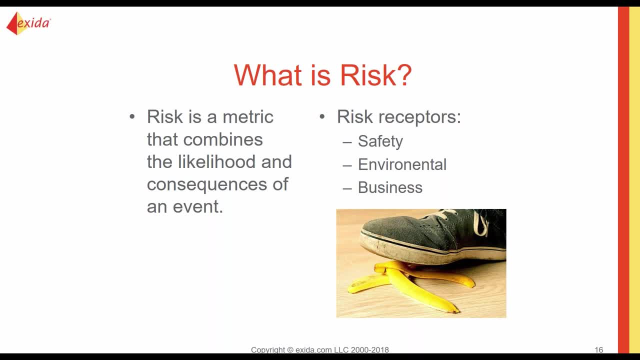 harmed Environmental risk, which is less important in robot applications. that's kind of interesting. So, for example, a robot against a than many of the others we look at. and then there's business risk. so if this part breaks, will it affect business? how much business loss will there be? so in 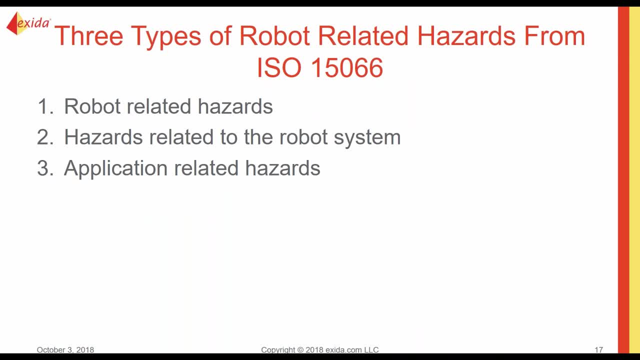 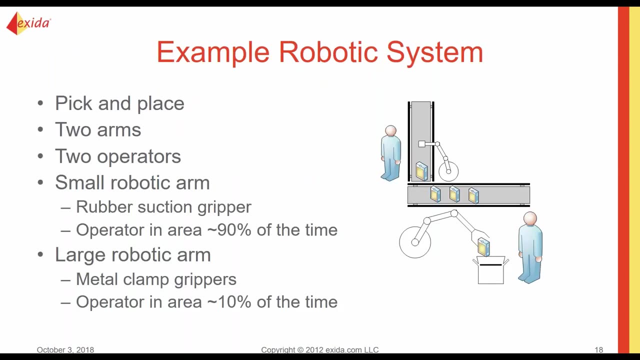 ISO 15066. there's three different types of robot related hazards that we're going to go through in these next couple slides. so there's robot related hazards, there's hazards related to the robot system and application related hazards. so to go through these hazards, we're gonna use this robotic example: robotic. 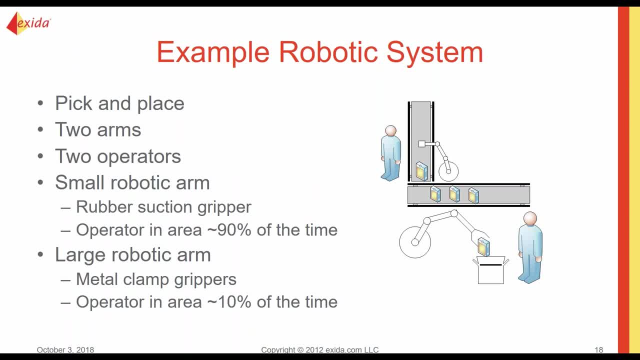 system to kind of demonstrate all the different hazards. so in this scenario we have a pick and place application where both the robotic arms are going to be picking up these boxes. you're gonna have two, two arms, two operators. the small one you see, the small one you see is the robotic arm. the robotic arm is the robotic arm. 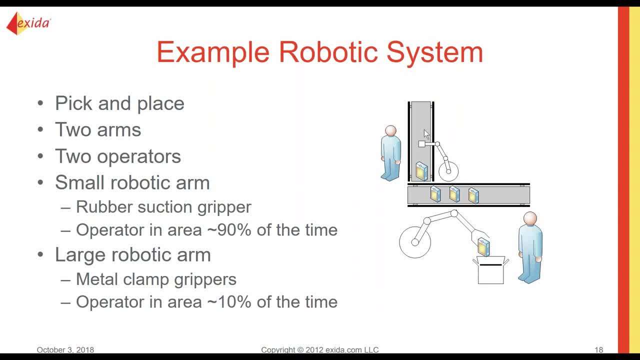 that's in the back over here. that's going to be a rubber suction gripper, so we'll talk about it more later, but it's gonna be a softer material, more rounded edges, and the operator here is going to be in the area for about 90% of the time. 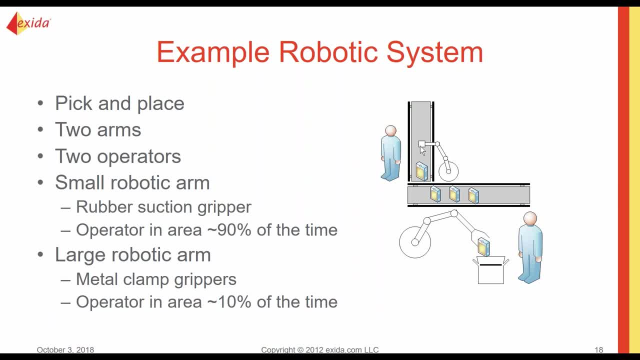 so it. he will be consistently working with the robot, though meanwhile the large robotic arm is going to have a metal clamp gripper and he's going to only be in the area about 10% of the time, so he's not working with the robot nearly as much. so first we'll talk about 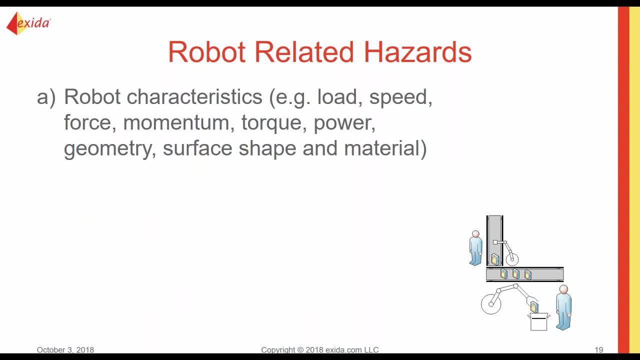 these robot related hazards. robot related hazards will include the robot characteristics. so load speed, force, momentum, torque power. so how much force is going to be exerted on the operator? as you can see this large one here, we'll say: this large one has three times as much force that can be generated from. 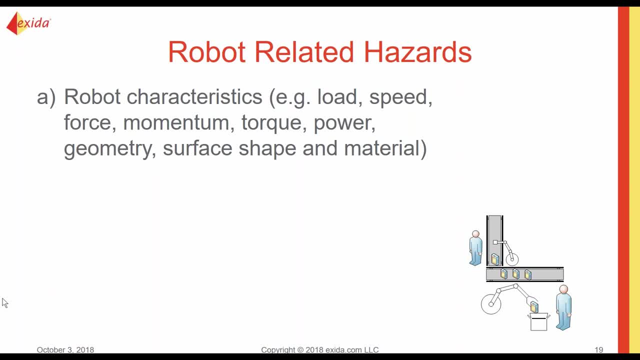 it compared to the smaller robot. so therefore there's going to be much greater hazard or risk probability or much higher risk because of the consequence being much higher for the, for the hazard. then we also have to look at the geometry and surface and the shape of the material. so, as we said, the 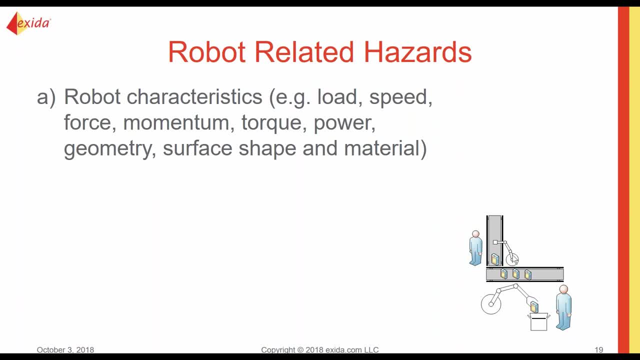 top one here. the small one is going to be a rubber suction gripper and the bottom one is going to be a rubber suction gripper and the bottom one is going to be a rubber suction gripper and the bottom one is going to be a rubber suction gripper. 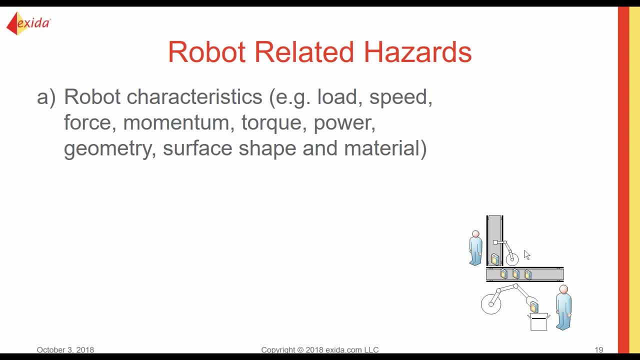 and because of that, or okay, so that's, that's more with the end piece. so these, we'll say, are like round arms, so they'll create a smaller, a larger surface area, which will definitely decrease the risk involved. because when you do look at the pressure, it's very important to look at the pressure of these, and when you 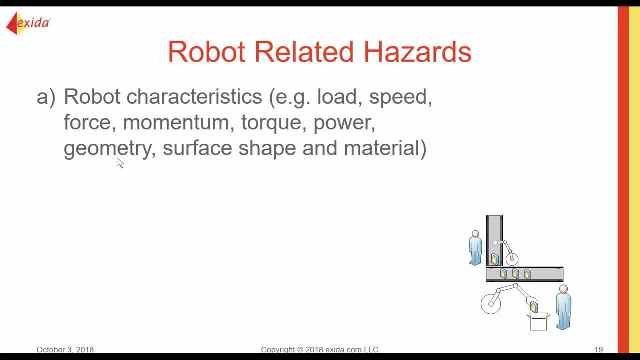 increase the surface area. you're going to decrease that, obviously, force over area. and so going back to the quasi-static, making sure that there's no quasi-static conditions in this robot. so operator location with proximity to the robot, so the top operator not very close, but he'll be working with that conveyor belt, it seems like so you. 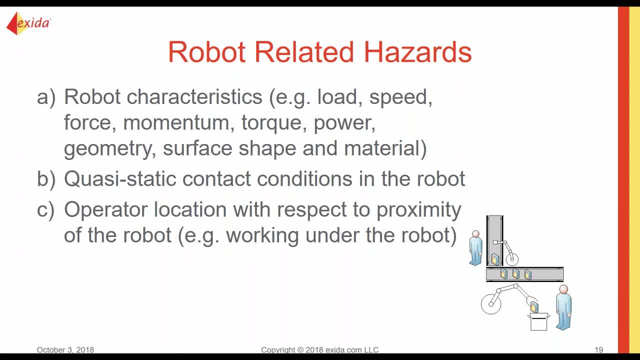 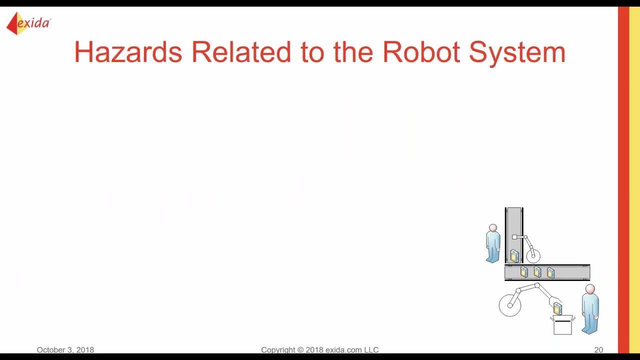 definitely have to take that into account is maybe his arms and hands will be very close to the robot and the guy on the bottom he's not nearly as close, so that's definitely good in a risk sense. next we'll look at the hazards related to the robot system, so this is going to take into account the end. 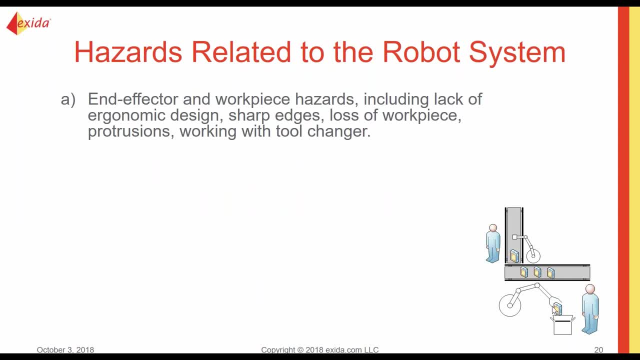 effector which I briefly touched on. so you have the middle gripper on the bottom- is going to have- it seems like it's going to have a Sharper angles and a harder material, so that's going to Increase the risk compared to this suction gripper on the top. 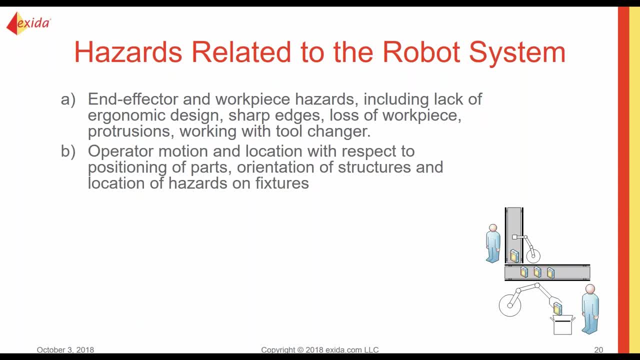 So then you also have to look at operator motion and location with respect to the parts. So is the operator with a conveyor belt on the top? how much is he going to be? How close is he going to be at the robot and how often is he going to be right next to the robot? 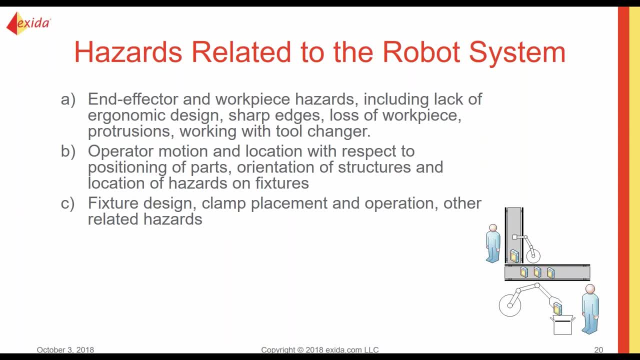 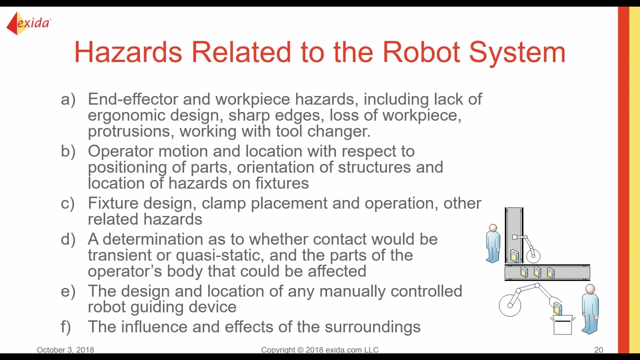 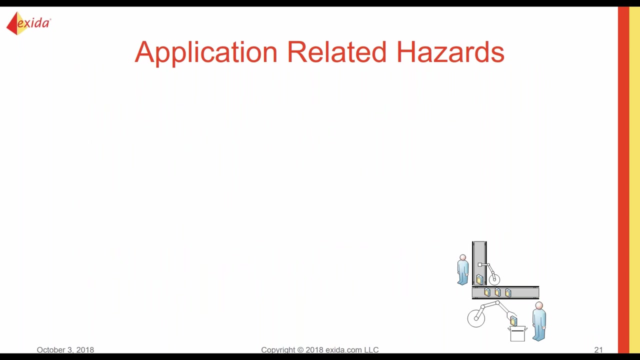 Fixture design. so maybe looking at that conveyor belt and any hazards can be evolved there Again, transient, quasi static. that's going to keep coming up because it's very important: Location or design location to any manually controlled robot guiding devices and Influence and effects of the surroundings. Okay and then so our last robotic hazard is going to be the application related hazard. 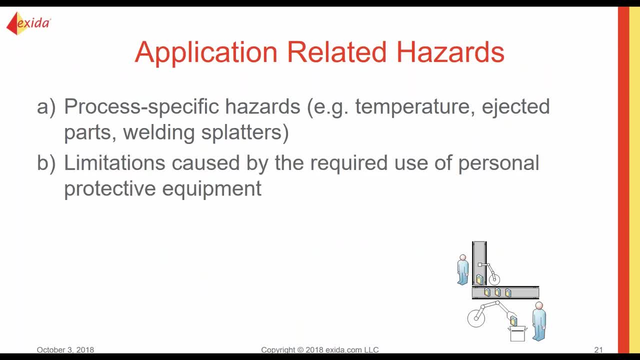 So we're going to look at process specific hazards, limits caused by the protect personal protective equipment and ergonomic design. So maybe you're going to look at surrounding processes, Maybe, so, welding splatters, Maybe there's something, a process going right next to it where there's could be like something, some sort of projectile coming from there that the operator needs to worry about. 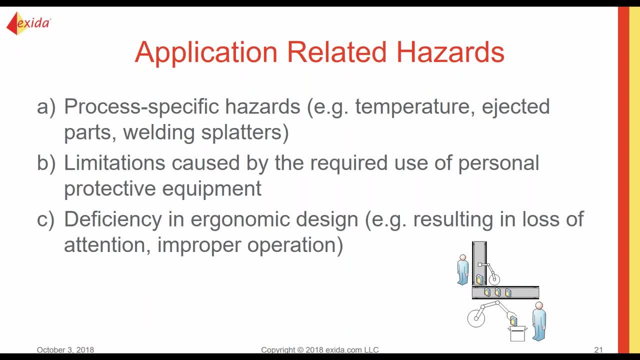 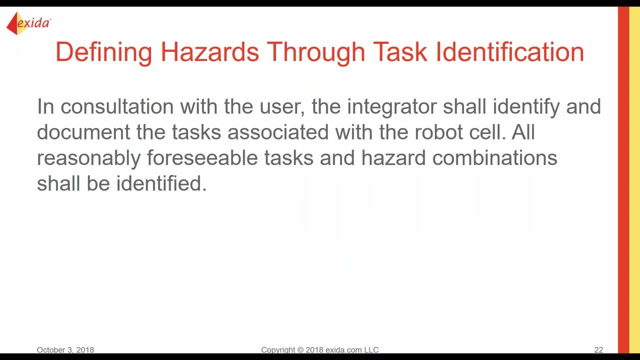 and Then also the personal protective equipment. So maybe these Looks like a blue suit is maybe restricting the operators motion and that could potentially bring up more hazards. All right, so defining hazards through task identification. So task identification is where you're going to work with. 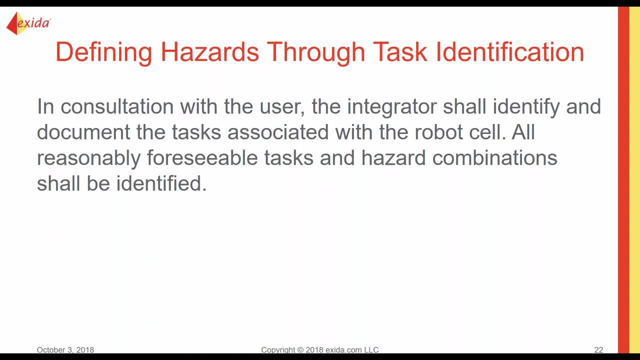 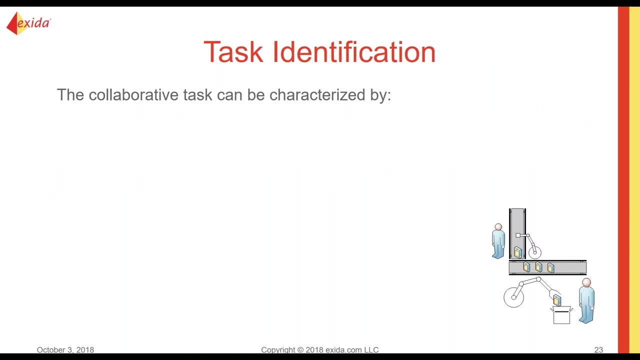 the end user to identify Additional hazards that can come up with the specific task that's being performed by the operator and How much he's going to be exposed to the robot. So collaborative task can be characterized by Quincy and duration of the robot, the operator presence in the collaborative workspace. 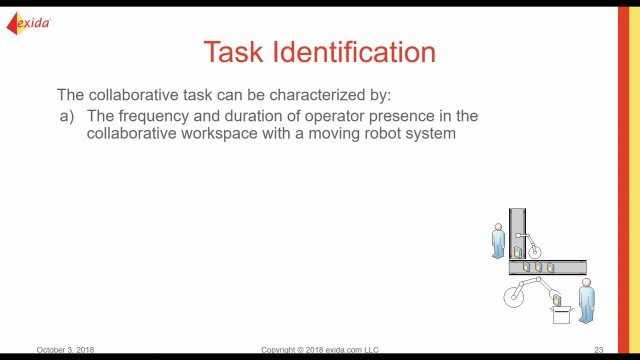 so we said earlier that the guy next to the large robot arm is only going to be there 10% of the time, So that'll greatly decrease the risk compared to the guy next to the small robot who's going to be there 90% of the time. So that definitely needs. 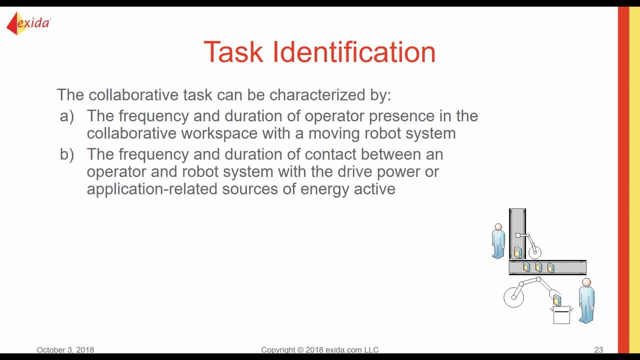 to be taken into account when you're looking at risk. And then so this is also the frequency and duration of contact. So if the guy, if they're in the area but they're not actually touching the robot, then that can also have an impact on the risk associated with the robot. 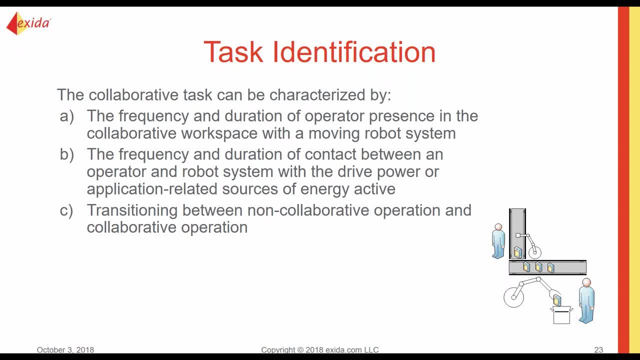 Transitioning between non-collaborative operation and collaborative operation. So are they on their way into the workspace? Is the robot system still going to be working? Because that could provide more hazards that maybe, on their way to the system, they could potentially. 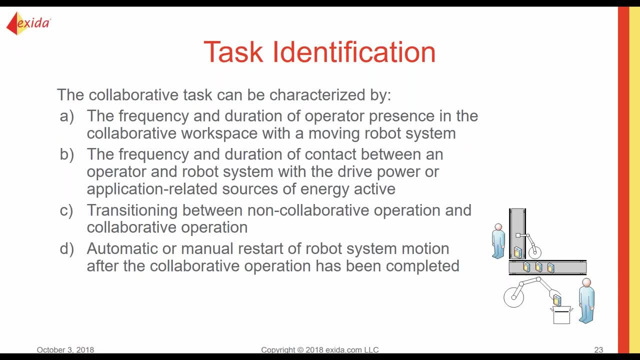 be harmed, Then automatic or manual restart. so if you have a manual restart, that could be just like an extra safeguard that could help mitigate the risk of the robotic system task involving more than one operator. so it's just extra risk that can happen when, naturally, when you have two operators in the same area and then in additionally. 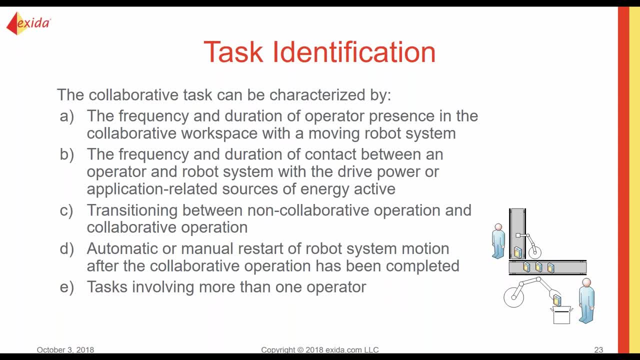 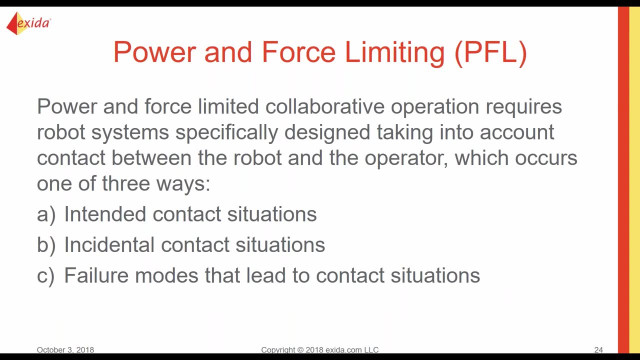 human error. with two people working together, maybe they create risks with each other and then any additional tasks within the collaborative workspace. okay, so now we're going to talk about power and force limiting. so often you're going to want to, through controller design, you're going to want to limit the amount. 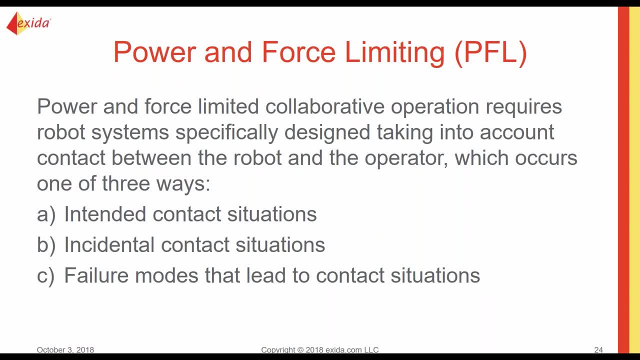 of power and force that can be in the robotic system, taking into account the various contact that can occur, you taking into account what body parts will be exposed to and what kind of contact situation. so you have these three contact situations. you have the intended contact situations, incidental contact situations and failure modes. 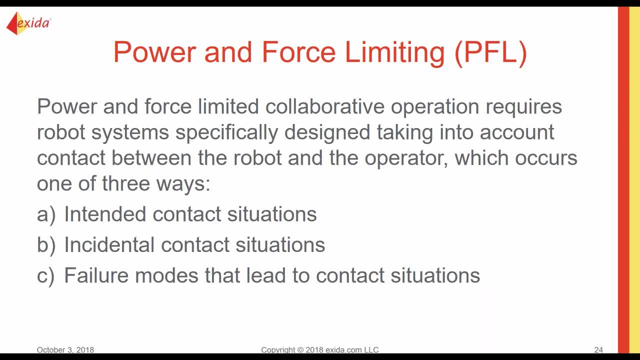 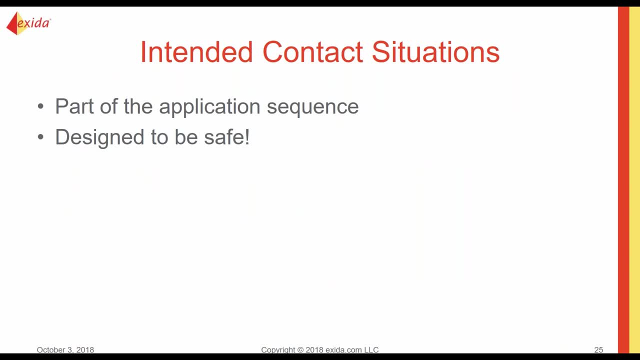 that lead to contact situations. so right now we're going to kind of briefly touch on these three. so the intended contact situations: they're going to be part of the application sequence and they're naturally going to be designed to be safe. so you might not need really any safeguards for those, because you know they're going. 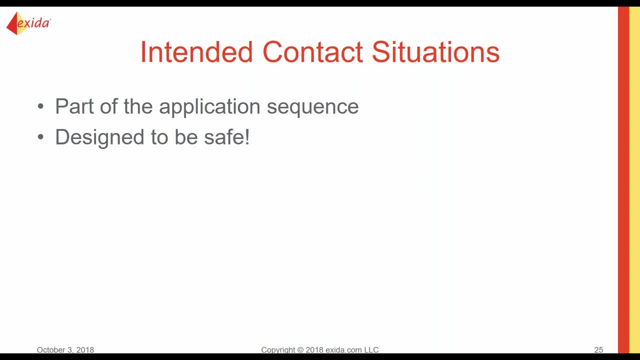 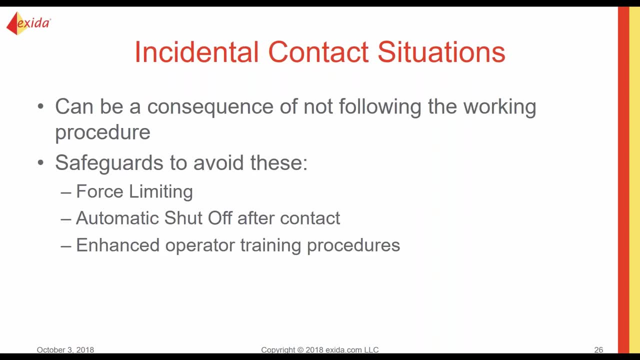 to occur and ahead of time you already designed it so that it won't create a hazard. then you have incidental contact situations. this is where a human error is going to come into play. so safeguards who avoid these would be using the force limiting so that when the contact situation 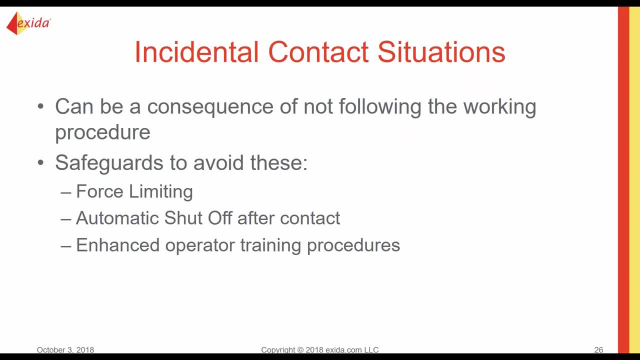 occurs to anyajuica function. you may needinity barriers for that to be able to locked in theuntil that you want to do safe guard andος because same drive to avoid data to an unintended body part, that it's not a significant damage. Then you can have automatic. 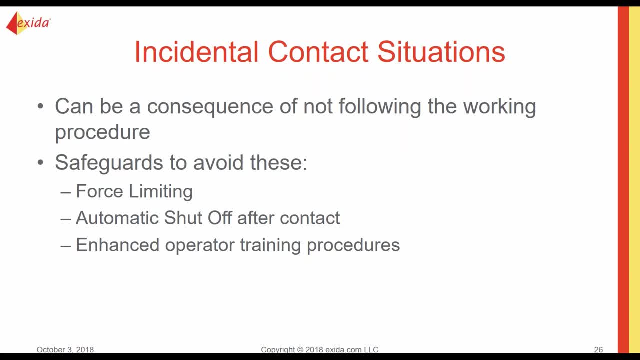 shutoff after contact. A lot of robots are going to be designed so that it'll immediately detect when it hits a body part or just another object and the robot's going to immediately shut down. And then, last, you can enhance operator training procedures so that you can hopefully avoid this. 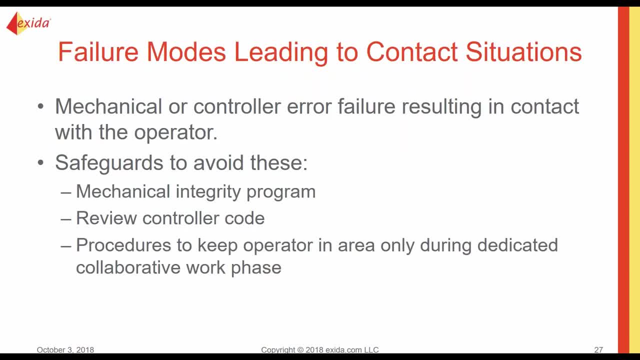 human error as much as possible. And then, lastly, we have failure modes leading to contact situations. So this is going to be either a mechanical or a controller error and it's going to result in contact with the operator. So, to avoid these, you're going to want maybe a mechanical. 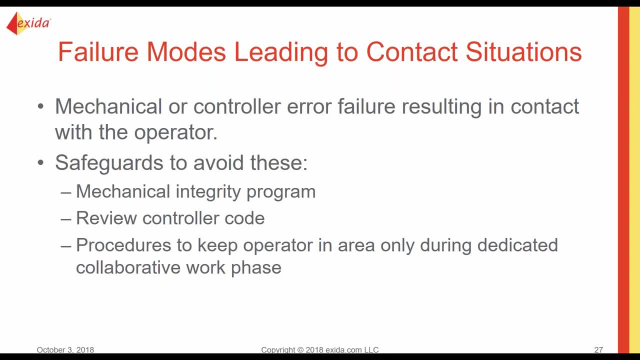 integrity program. So that'll be making sure that the mechanical components are not worn out and they're not going to fail. They're not going to have random failures that happen, or at least you can decrease the risk of this happening. And then you also might want to review the controller code so that the robot 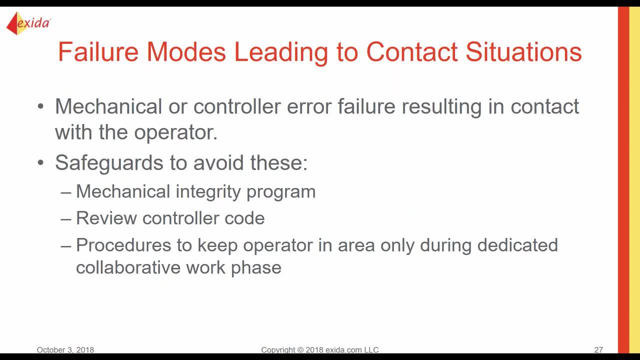 doesn't go out of spec and do something that is unintended. And last, you're going to want procedures to keep the operator in the area only during dedicated collaborative work phase, so that when these do happen, they don't actually impact the worker or injury. 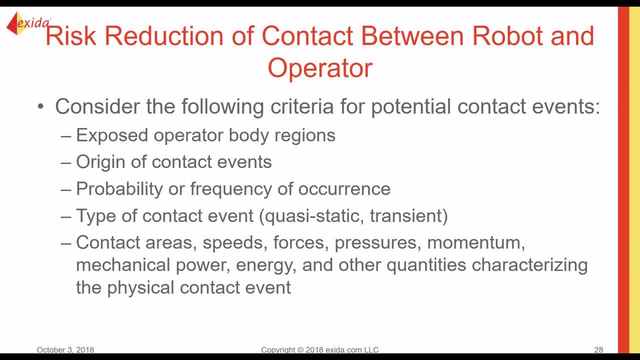 All right. so now we want to talk about risk reduction with robot contact. So you want to consider the following for potential contact events: exposed operator body regions. So you want to, at all costs, you want to eliminate the possibility for the operator being struck in the head or the face. 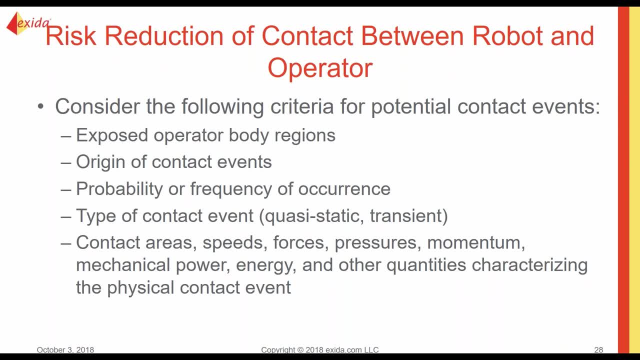 area And when you're looking at different body parts- we're going to talk later about biomechanical limits, And so different body parts can tolerate a certain amount of forces and pressures. You also want to look at origin of contact events, So where are they occurring? 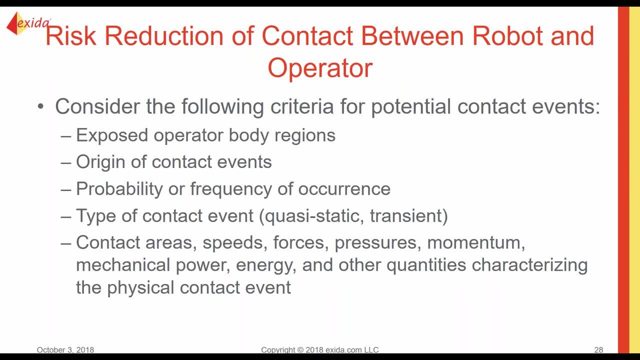 and probability or frequency of occurrence. And then you want to talk about quasi-static or transient again, because the transient allows for twice as much of a tolerable force to occur, And then your property functions will be very, very important. So you're going to want to look at the 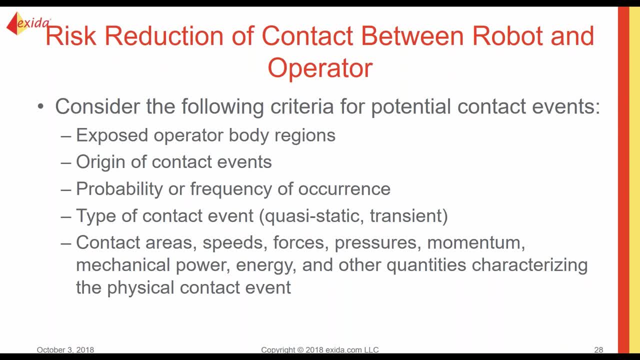 Last, you want to look at contact areas: speeds, forces, pressures, momentum, So things that will increase the force and increase the consequence when an operator is struck by the robot or part of a robot system. All right, so steps to achieving robot risk reduction. 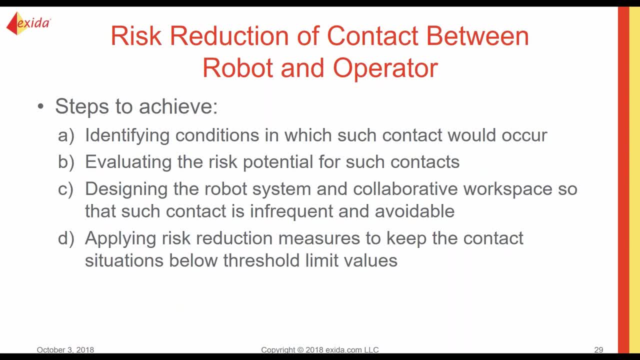 So first you want to identify the conditions in which contact could occur, Then you want to evaluate the risk potential for such contact events. So you want to see the likelihood of each thing happening, taking into account human error, amount of time that the operator is in the area. 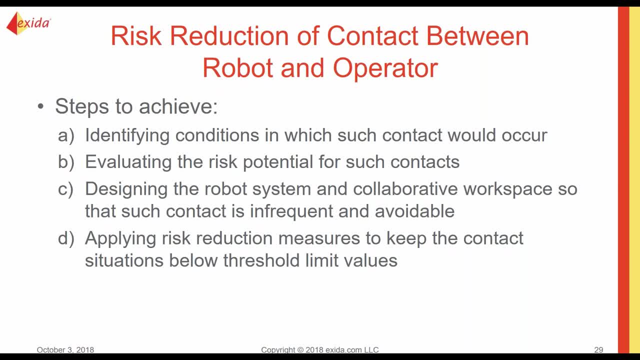 And then you want to look at the consequence and the force that's on the robot, And so then you want to look at designing the robot and collaborative workspace so that such contact is infrequent and avoidable. So this is kind of before. Before the robot's even operating, you want to make sure that it's designed with safety. 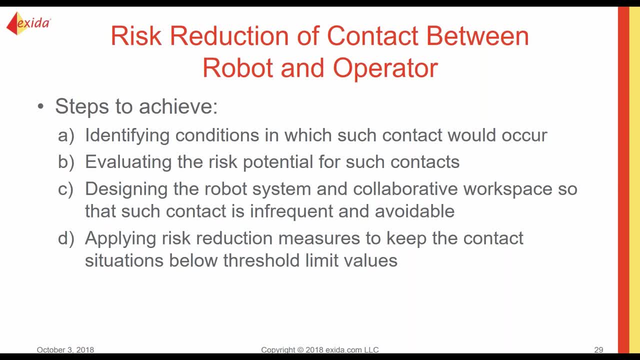 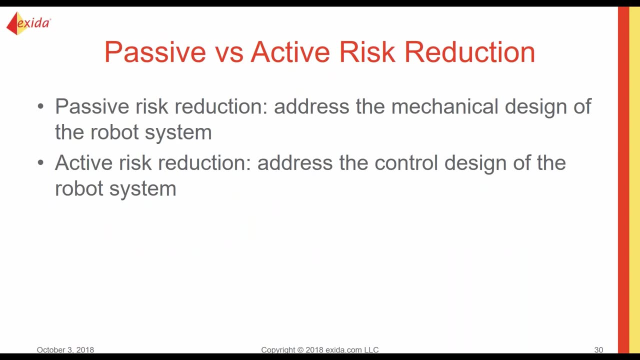 And then, last, applying risk reduction measures to keep the contact situations below threshold limits. So maybe changing your controller coding so that the risk is mitigated as much as possible. All right, so there's two different kinds of risk reduction, So we're going to touch on each of these. 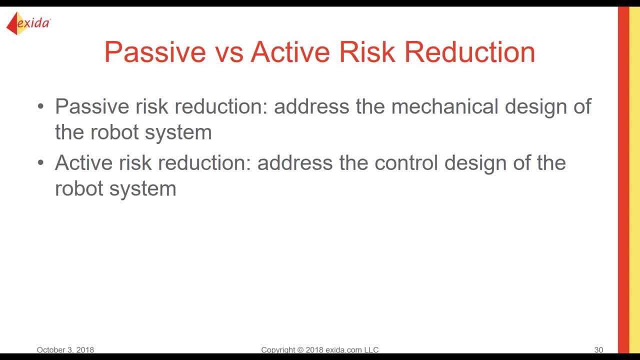 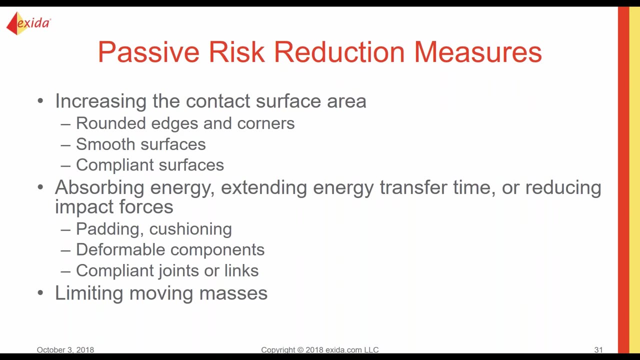 There's passive risk reduction. It addresses the mechanical design of the robot system and the active risk reduction will address the control design of the robot system. So, passive reduction, mechanical design, So you want to look at increasing contact surface area with rounded edges, smooth surfaces, compliant surfaces, because this will decrease the pressure that is gone, that is on the operator, and will avoid like cutting and 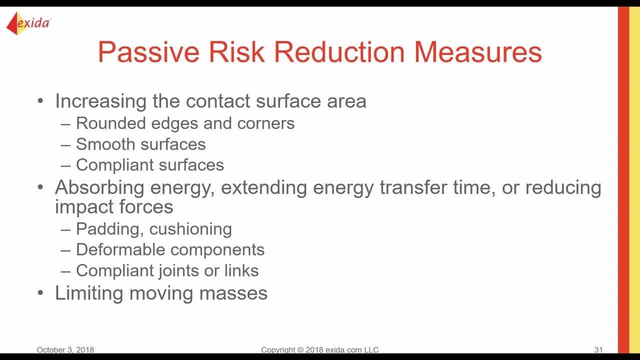 So then you want to look at absorbing energy, extending energy transfer time or reducing impact forces, So adding padding and cushioning. So maybe that rubber gripper design might be more effective than the clamp design, if it's possible to use that in your application. 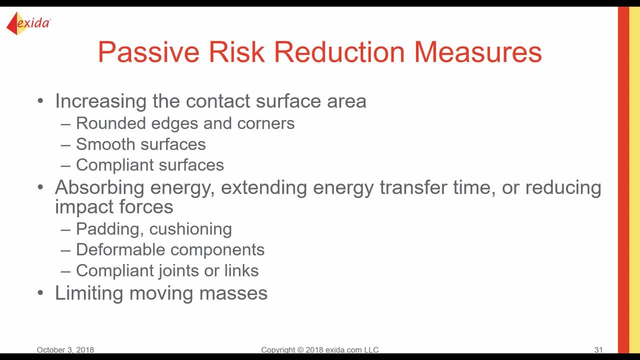 And then deformable components and compliant joints or links. Last you have limiting moving masses, So just kind of looking at the different components. So then you want to look at absorbing energy, extending energy transfer time or reducing impact forces. So that's kind of making the design simpler so that there's less hazards in the area and less hazards for the operator to pay attention to, so that they can acknowledge them and avoid them. 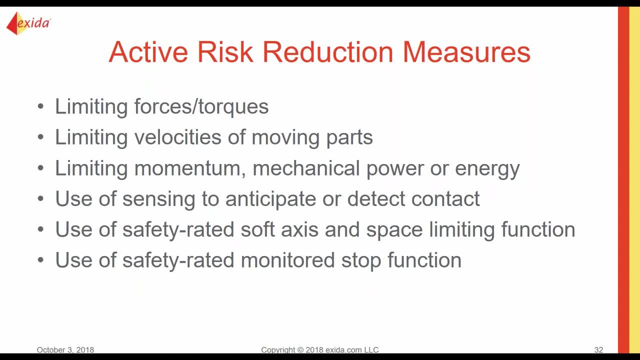 Then we have active risk reduction measures, which is your controller adjusting your controls. So you want to. we talked about force limiting, So limiting those forces and torques that are allowed in the system. So you want to. we talked about force limiting, so limiting those forces and torques that are allowed in the system. 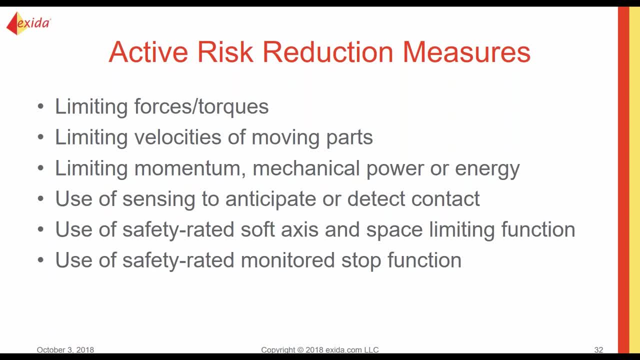 So you want to. we talked about force limiting, so limiting those forces and torques that are allowed in the robot design. So you want to. we talked about force limiting, so limiting those forces and torques that are allowed in the robot design, Limiting velocities and moving parts. 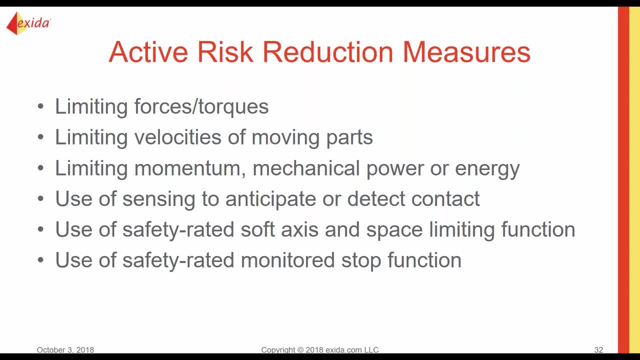 So that will influence the force, but it will also influence the operator's ability to get away from the hazard. but it will also influence the operator's ability to get away from the hazard. Then we have limiting momentum, mechanical power or energy. So that's also has to do with your force. 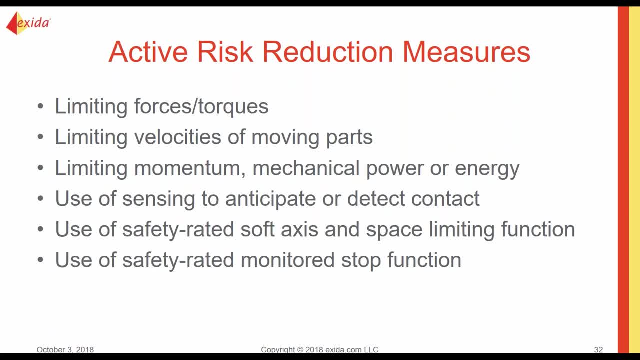 And then you want to look at using sensing to anticipate or detect contact. So a lot of times you can make it so that we talked about a robot being able to start at, stop at impact of an operator or just another object. You can also design it so it'll detect an operator in the area and stop before the contact. 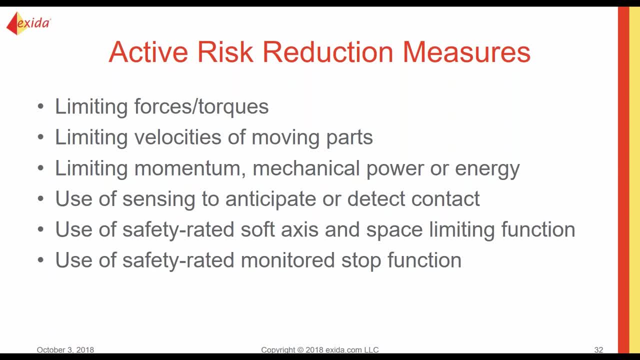 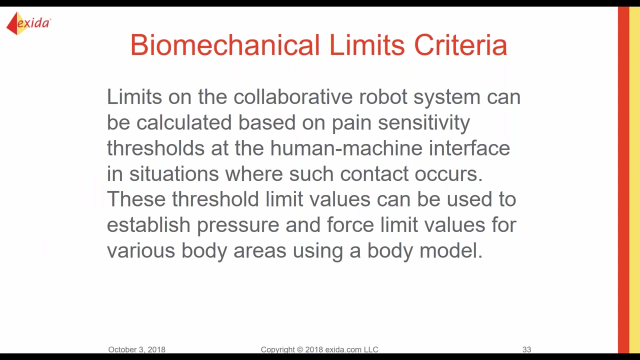 even happens, Then using safety rated soft access and space limiting function, so making the range of the robot arm smaller, so that there's just less of a radius for the robot to create a hazard, and then safety monitored stop function. Now we're going to talk about biomechanical limits criteria. 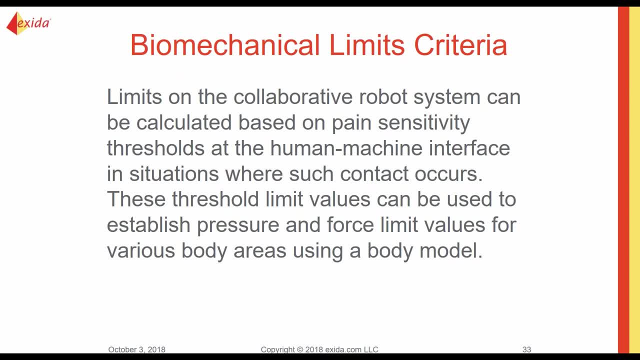 We briefly talked about this before, and so then we'll go a little more in depth. These are limits Based off of pain sensitivity of each body part. it'll literally list everything from your head and your ears and face to your feet. It lists tolerable pain thresholds for each of these, in both quasi-static and transient. 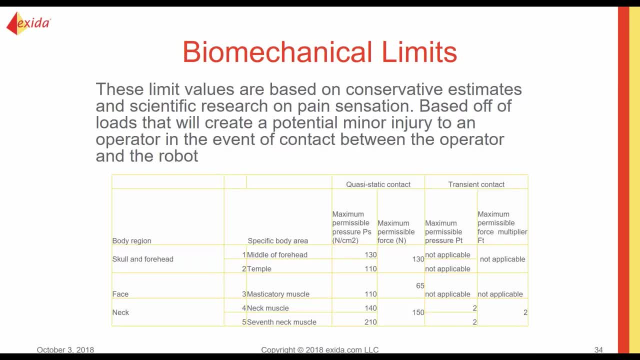 contact. So here's kind of just a little snippet of that biomechanical limits chart and so you can see here the skull and the forehead and the face are going to want to be avoided at basically at all costs, and that's why they don't really change anything for transient contact versus. 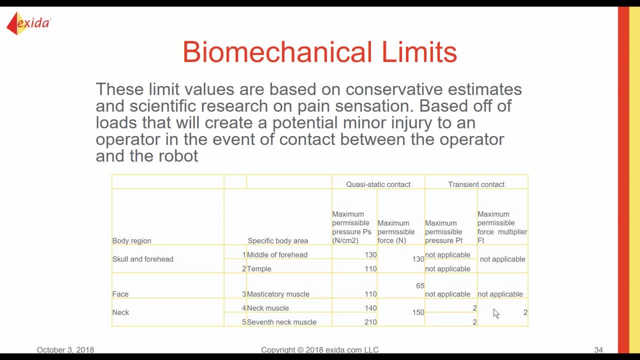 quasi static contact. but when you get into the other body parts, everything from the neck down is going to be the transient contact is going to be doubled for a tolerable pain threshold. so it's much more. you definitely want to see transient contact compared to the quasi static contract contact when 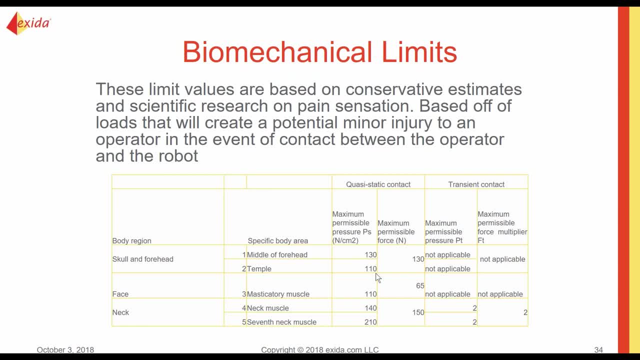 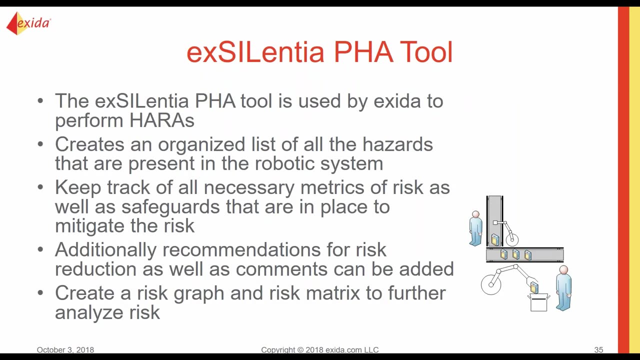 contact needs to occur. okay, yeah, so these are based off of conservative estimates and scientific research of pain sensation. all right, so now I'm going to. we're going to talk about the epigenetics of pain sensation, and then we're going to talk about the epigenetics of pain sensation, and then we're going to talk about the. 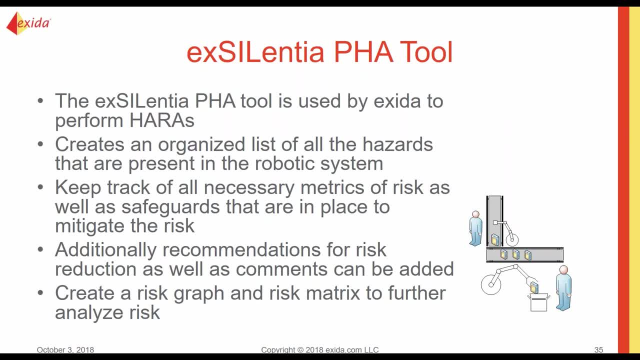 epigenetics of pain sensation. and then we're going to talk about the excellent PHA tool. so it's used by Exeda to perform the hazard analysis and risk assessments and it'll just create a very organized list of all the hazards that are present in the robotic system so that you can see all of the 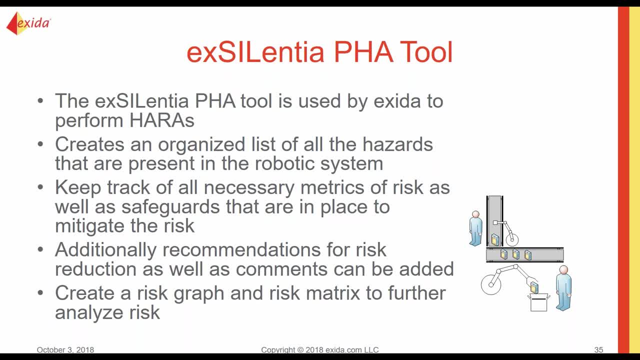 likelihoods, the consequences, safeguards, recommendations. so it effectively will just organize everything so you can look at your system as a whole and see where you can address risk and to reduce risk of the overall system most effectively and cost effectively. oh, whoops, yes, so actually now I'm going to take you to. 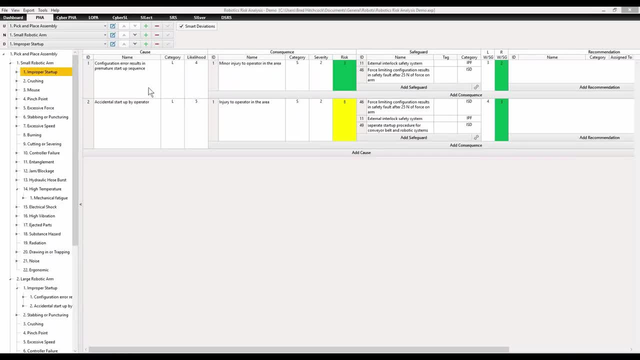 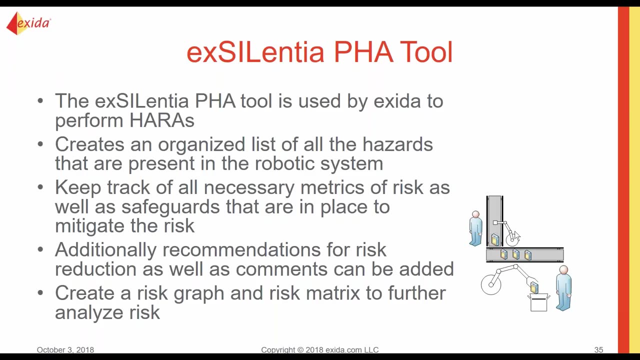 the excellent ship PHA tool. so in this example we have we're going to use the same. we're actually going to say use the same system as we were using before, with the small robotic arm and the large robotic arm and all the same conditions I talked before, with the operators being in the area 10% of the. 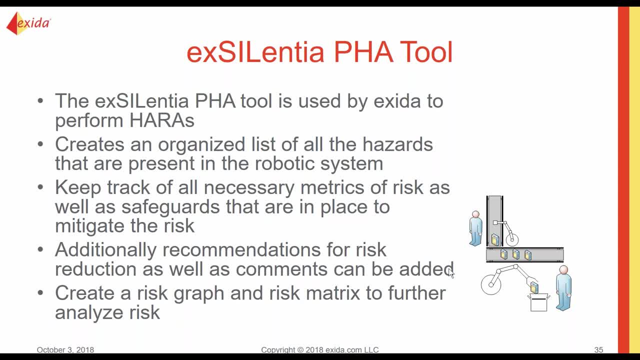 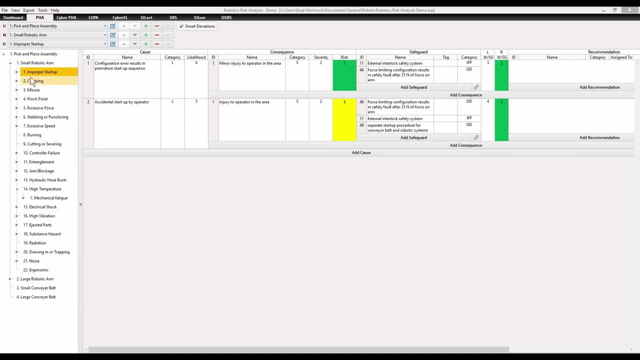 time for the large robotic arm. 90% for the top, all right. so yeah, let's so for the small robotic arm, we're first going to look at improper startup. so we have two different causes for improper startup. and there will be a configuration, configuration error that's going to result in the premature startup. 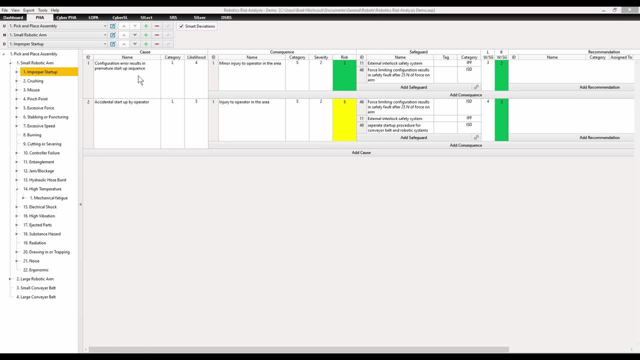 or there's going to be an excellent accidental error by the operator. so the likelihood of these, you're going to see a lot more of these with accidental startup by the operator because you have to expect human error to occur. so we're saying that this is going to be 10 to the negative, 1 to negative, 10 to the. 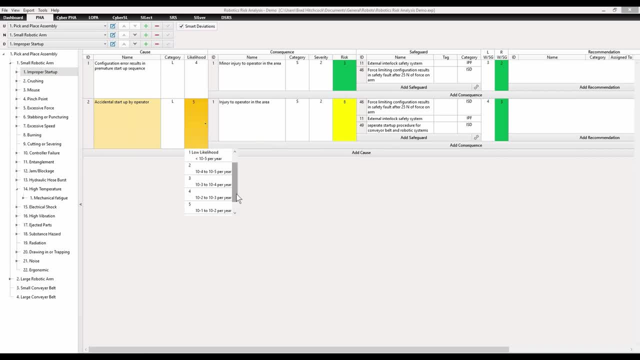 negative 2 per year, which is you could even go even higher than that, considering it's a decent likelihood of an operator starting up the system, while the configuration error, we're going to say it's down one magnitude- 10 to the negative 2 to 10 to the negative 3 per year- and we're going to say the same. 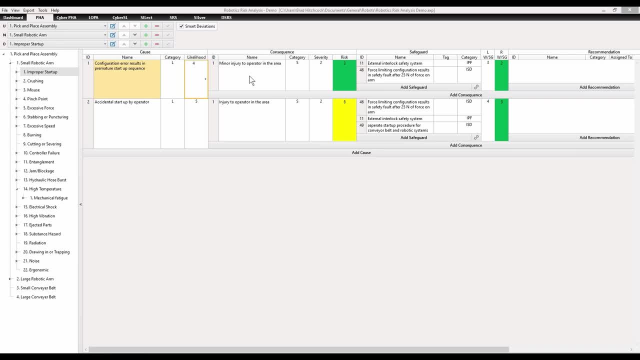 consequence occurs for the width of these, so minor injury to the operator in the area and they're going to have the same severity. so we're going to say that's going to be recordable injury, so maybe like a hand gets pinched, but we're not going to say there's lost time because of this. and, as you can see, the 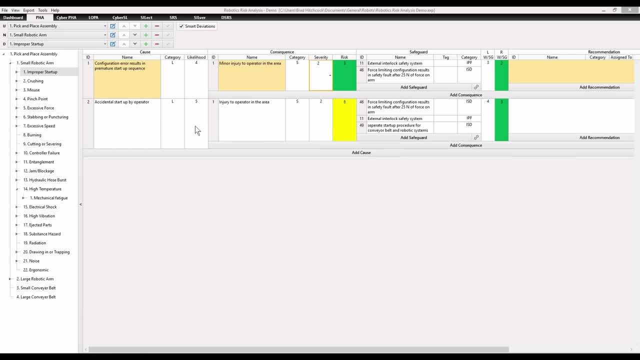 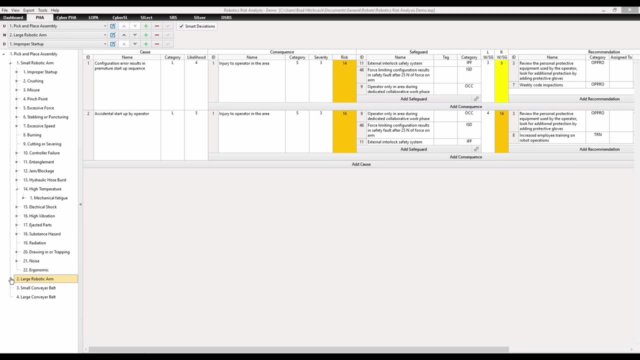 risk for the accidental startup because it's a lot more- it's like more likely by a full magnitude. so we're going to say the risk is much higher than that of the configuration error. so we're going to compare this to the large robotic arm improper startup. so the likelihood of those is going to be the same because 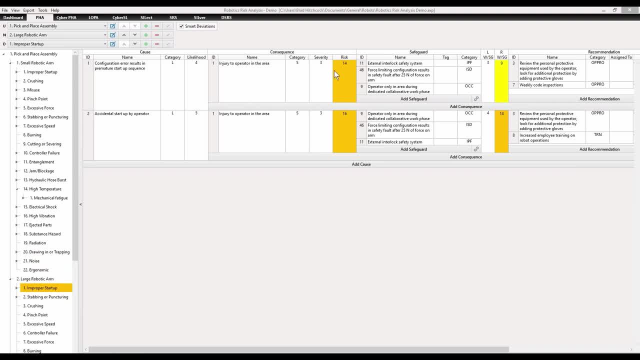 it's the same cause, but the consequence is we're going to say that the severity goes up to a lost time injury because, as we said before, we're going to say there's three times as much force that's going to be exerted on this robot. so you could see, maybe like 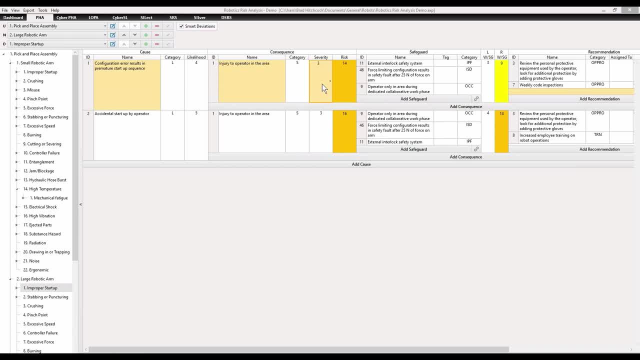 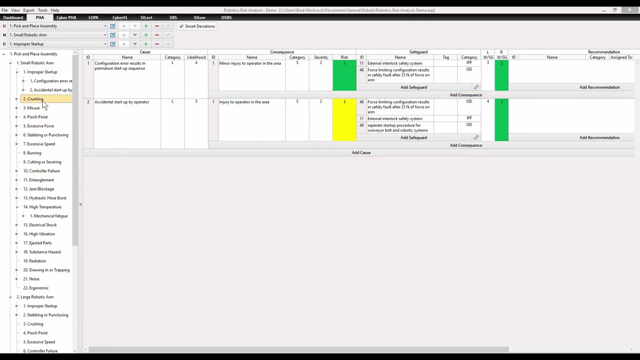 potentially a bad bruise or even a broken hand, and so that'll increase your risk by a good amount. I'll go from to 16 and 14, from eight and three, all right, so now we're going to talk about, we're going to go to crushing, so 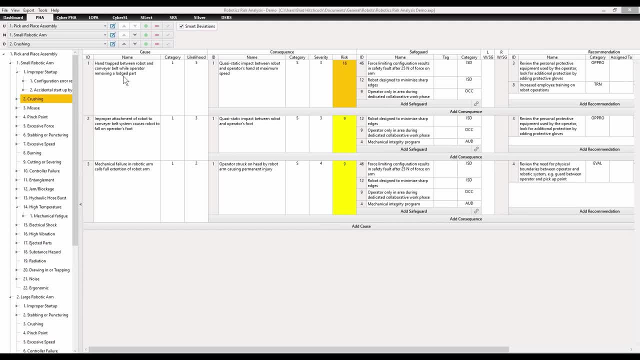 this has three different causes. we'll just talk about this top one, because I want to use this one just to talk about safeguards and recommendations. and so the cause is going to be hand-trapped between the robot and the conveyor belt while the operator is removing a lodged part, so you can see a operator, a lot of. 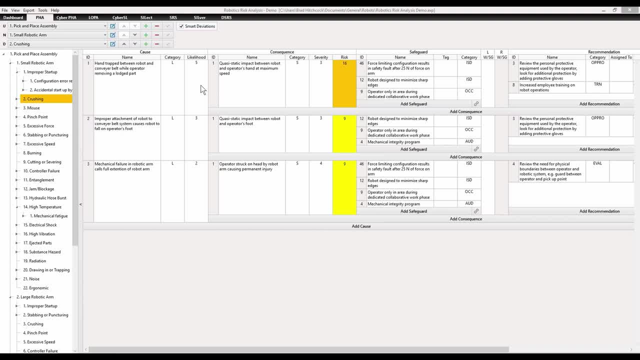 so you can see a operator. a lot of times you'll have parts stuck in a conveyor belt and an operator's natural instinct will be to try to remove that. so we're going to give that a likelihood of five, and the contact the consequence will be, we're going to see 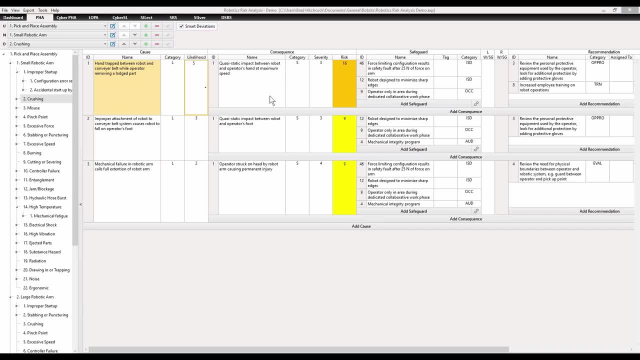 quasi-static impact between the robot and the operators hand at maximum speed. so it's kind of like a worst case and we're going to say that's a three, so a lost time, injury, and so it's going to be a pretty high risk. but you can see. 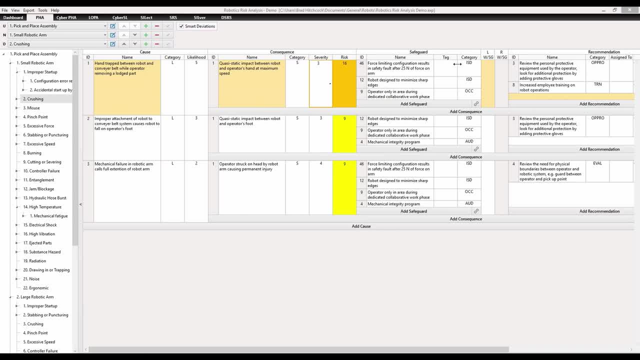 see, here we have safeguards, so we're going to say that the robot has force limiting configurations, resulting in a safety fall after 25 Newtons of force on the arm. there's also going to be a robot designed to minimize sharp edges and the operator is only going to be in the area during dedicated collaborative work. 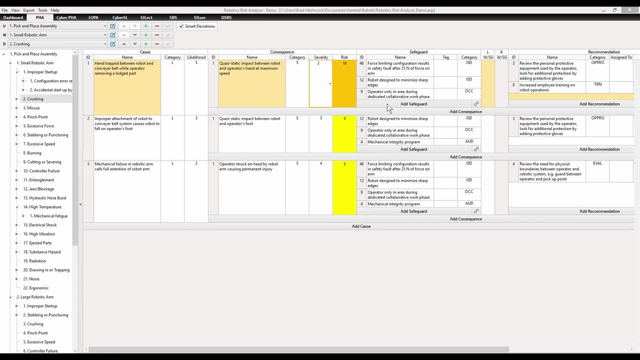 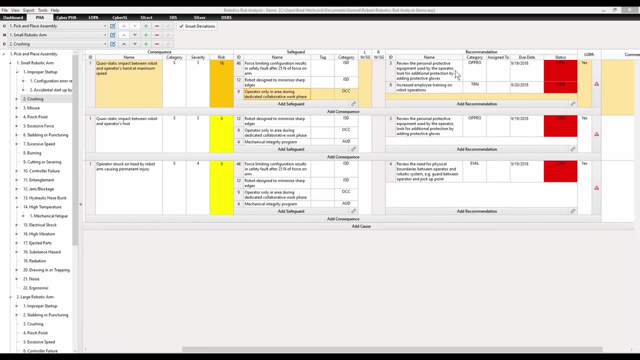 phase. so for this one it's actually the operator only in the area. since we said it's 90% of the time, that's not going to be as big of a risk reductor, so after that you can also add recommendations for additional things that can be added. 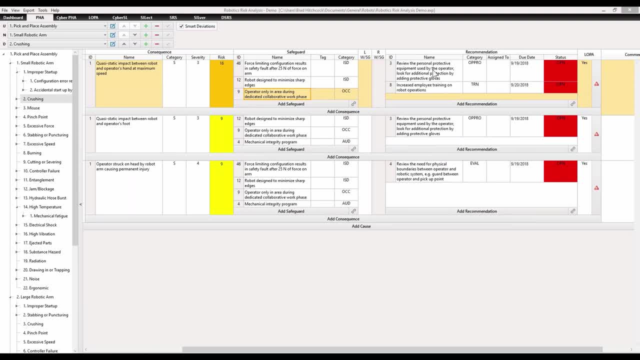 to mitigate the risk. so this could be a review of the protect personal protective equipment used by the operator may be adding gloves to further protect them and then increasing employee training on the robot operation you. so these are just like additional things that you can like, suggest, and right now. 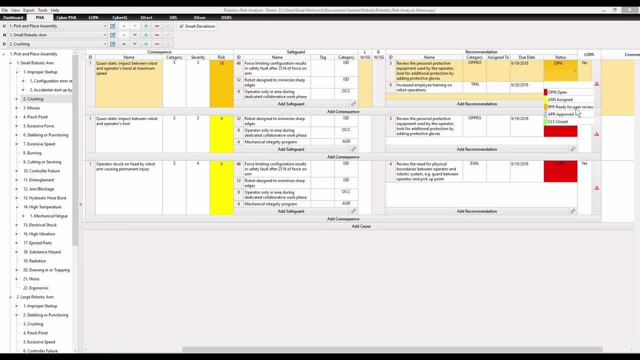 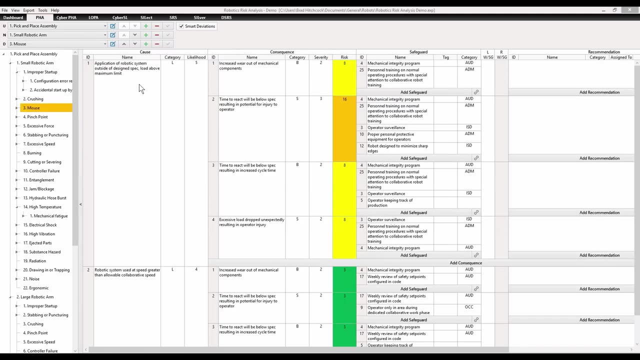 they're open, but you can say that they're assigned or ready, approved, ready for peer review or closed. so the last deviation we're going to talk about is misuse. so we'll look at this one application of robot system outside of design spec. the load is above the maximum limit, so you can see here. that the robot has force limiting configurations resulting in a safety fall after 25 Newtons of force on the arm. there's also going to be a review of the protect personal protective equipment used by the operator. may be adding gloves to further mitigate the risk reduction. you 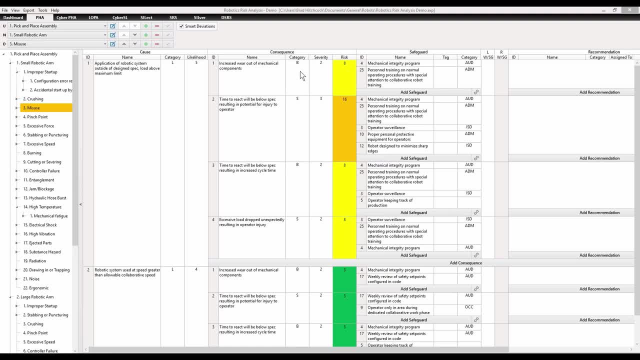 there's going to be four different consequences, and this one's actually going to include business consequences. so the first one is going to be increased wear out of mechanical components, and that's going to be a we're gonna see a business consequence out of this. the business consequences tend to be a lot. 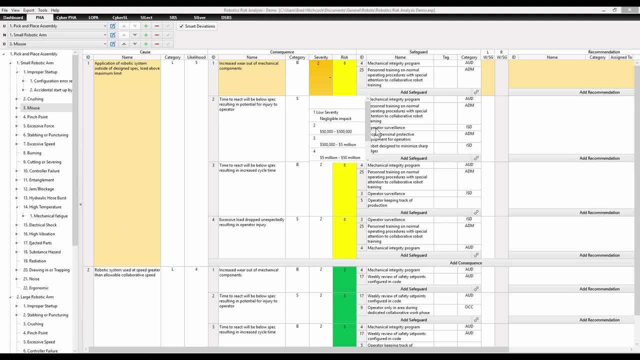 lower than the safety. so just to get a two, you need fifty thousand to five hundred thousand dollars in damage. so just having this two sort of implied is that we're maybe replacing the entire robot just to create a risk of eight. And then for the business you can also include safeguards, and the safeguards are a lot of. 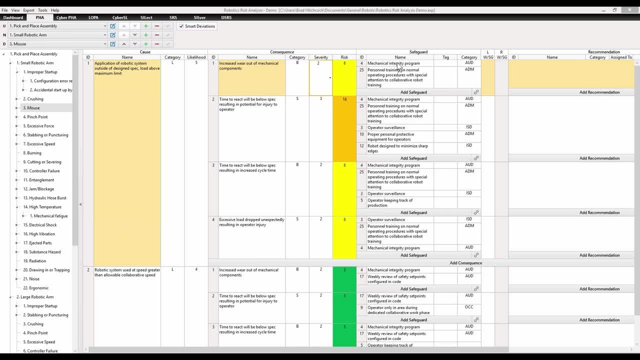 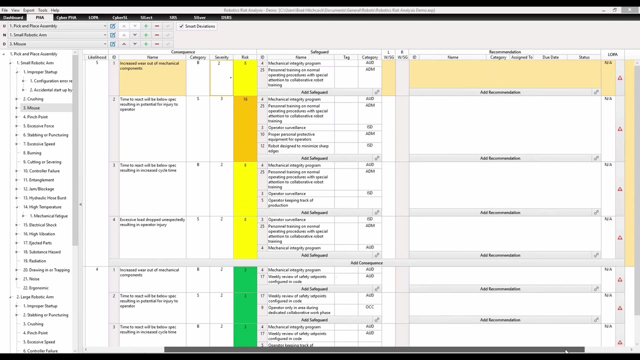 times the same one as the safety safeguards, just because having a mechanical integrity program will increase the will improve like the wear out of the components, but it'll also improve the safety of the operator. Same with personnel training on operating procedures. And then there's no recommendations right now, but obviously you can add recommendations. 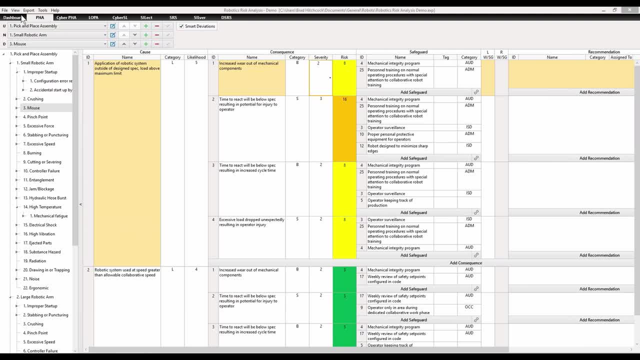 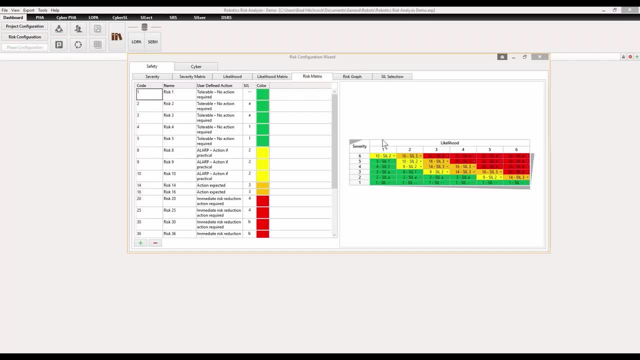 on to that, Okay and then. so the last thing I'm going to show you on the Excellencia is the. I'm going to show you a risk matrix, So this will show you. you can kind of adjust these values to be tailored to your system. 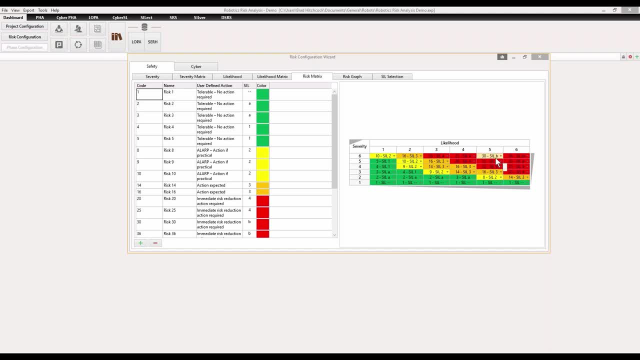 and you can see that the the ones over here. so when you get a risk score of 20 to 30, you're going to those are going to be like high priority and you're going to want to address those before you even start operating the system again. 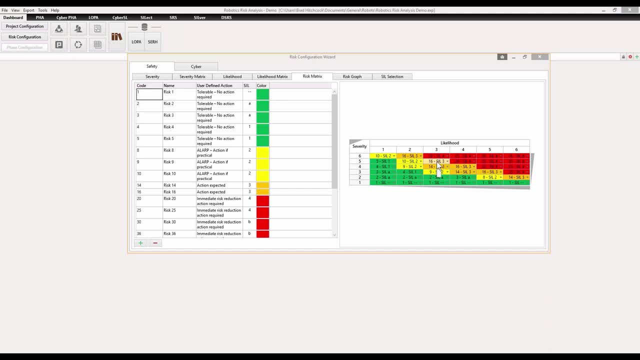 While when you get into these orange, it's also high priority, definitely wants to be addressed soon, but once you get down into the green it's lower priority. but they definitely are things you want to address. Same with the yellow. you know those are things you want to address, but you want to. 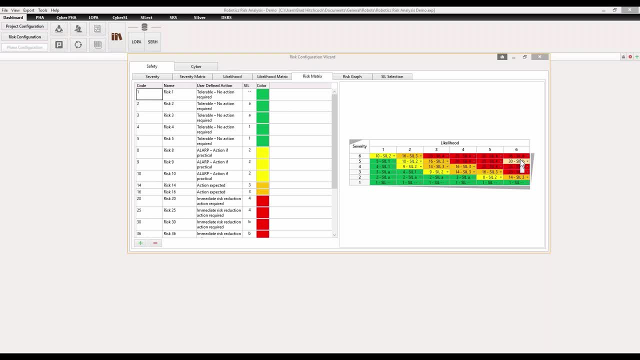 take care of these red ones first and those will help you create the biggest risk reduction And just most effectively reduce risk of the system as a whole. So it kind of gives you a gauge of where your priorities should be with when you're trying.